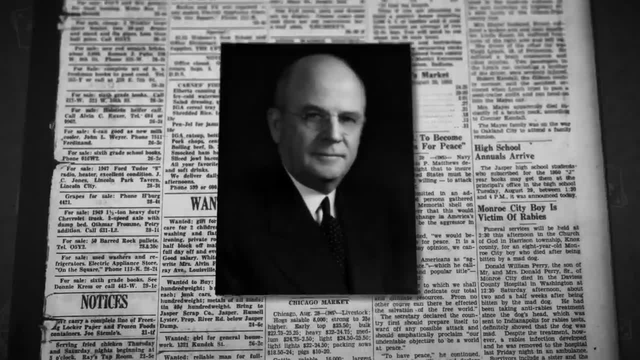 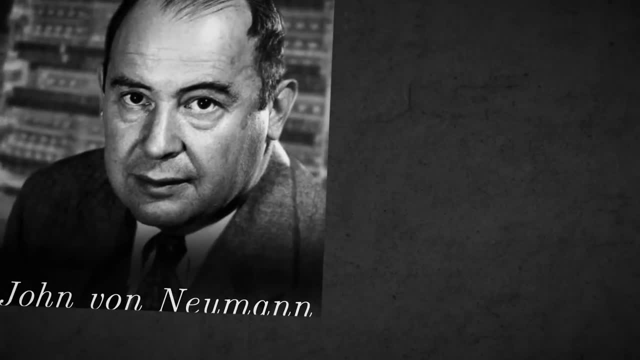 Soviets while they were still ahead- In the words of Navy Secretary Matthews- to become aggressors for peace. John von Neumann, the founder of Game Theory, said: If you say why not bomb them tomorrow, I say why not bomb them tomorrow? If you say why not bomb them tomorrow, I say: why not bomb them tomorrow? I say: why not bomb them tomorrow? If you say, why not bomb them tomorrow, I say, why not bomb them tomorrow? I say: why not bomb them tomorrow? 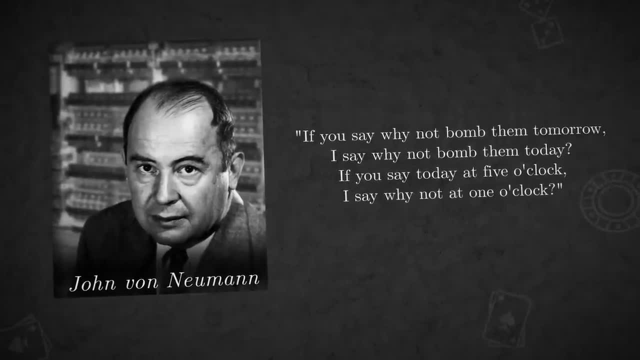 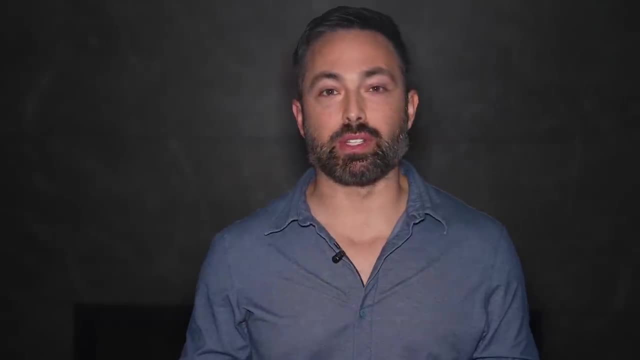 But in fact they did today. If you say today at the 5 o'clock later tomorrow, I say why not at the 1 o'clock? Something needed to be done about nuclear weapons, and fast. In 1950, the RAND Corporation- a US. In 1950, the RAND Corporation, a US-based think tank. 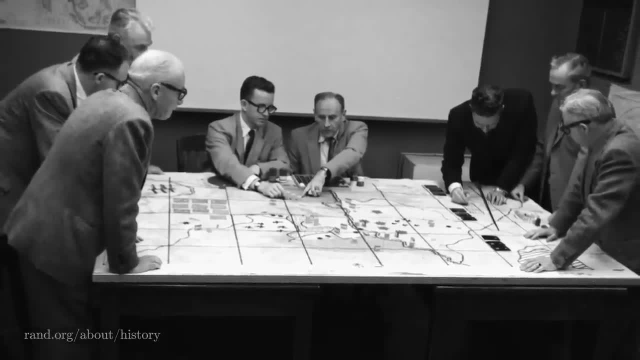 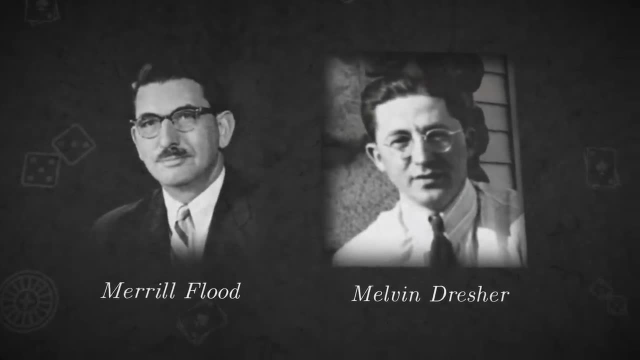 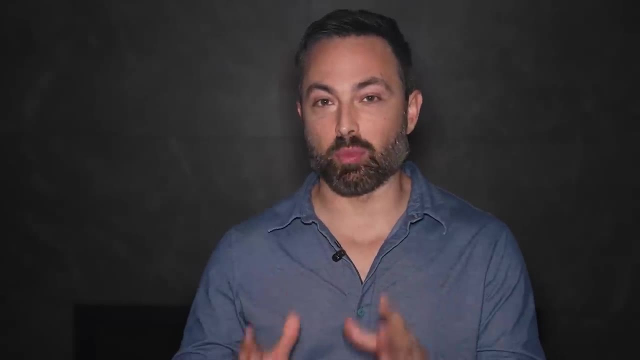 was studying this question, And that became Game Theory. This RAND was mainly focused on absurdity such as the ground, unbeknownst to them at the time, closely resembled the US-Soviet conflict. This game is now known as The Prisoner's Dilemma. so let's play a game. 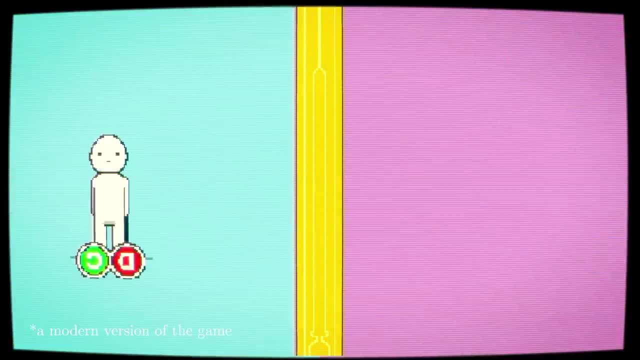 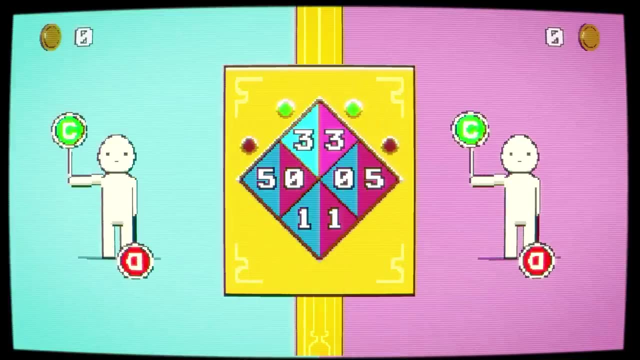 A banker with a chest full of gold coins invites you and another player to play against each other. You each get two choices: You can cooperate or you can defect. If you both cooperate, you each get three coins. If one of you cooperates but the other defects, then the one who defected gets five coins. 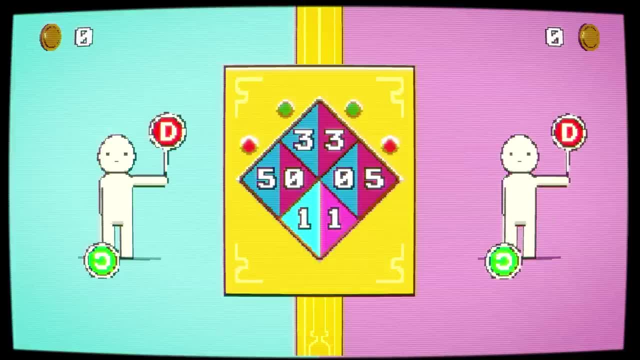 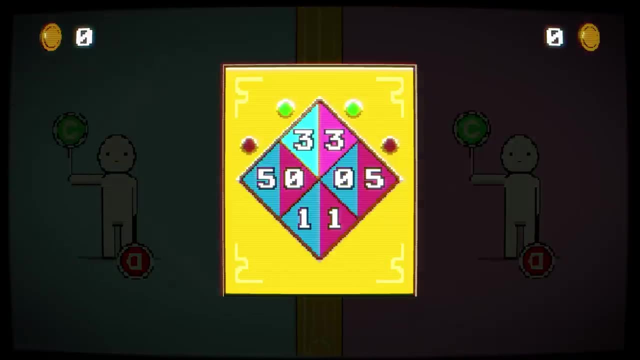 and the other gets nothing, And if you both defect, then you each get a coin. The goal of the game is simple: to get as many coins as you can. So what would you do? Suppose your opponent cooperates? then you could also cooperate and get three coins. 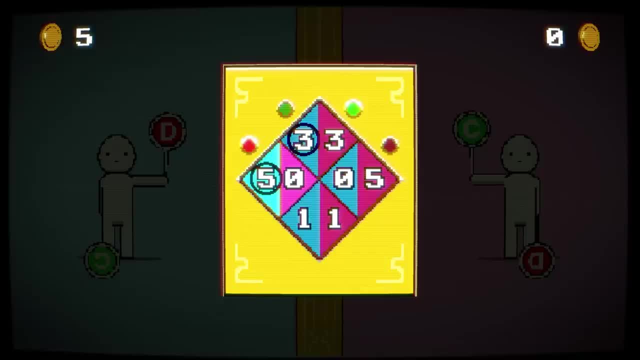 Or you could defect and get five coins instead. So you are better off defecting. But what if your opponent defects instead? Well, You could cooperate and get no coins, or you could defect and at least get one coin. So, no matter what your opponent does, your best option is always to defect. 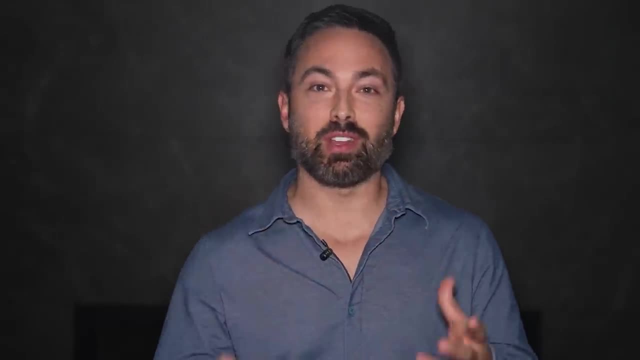 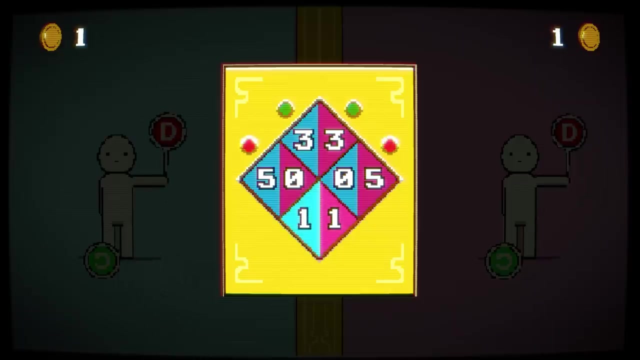 Now, if your opponent is also rational, they will reach the same conclusion and therefore also defect. As a result. when you both act rationally, you both end up in the suboptimal situation, getting one coin each when you could have gotten three instead. 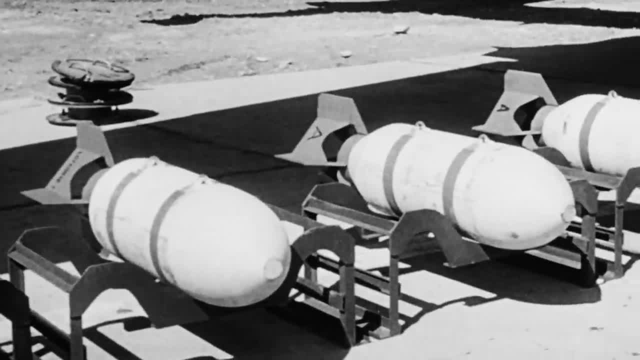 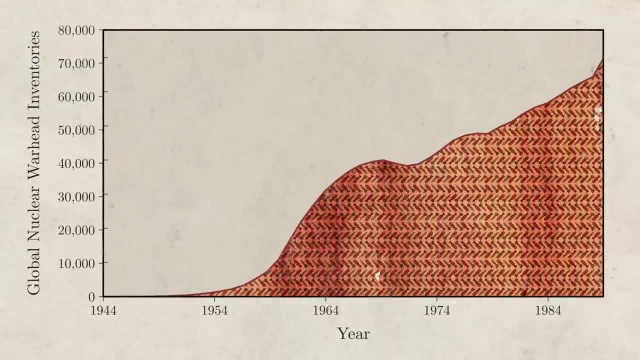 In the case of the US and Soviet Union, this led both countries to develop huge nuclear arsenals of tens of thousands of nuclear weapons, each more than enough to destroy each other many times over. But since both countries had nukes, neither could use them. 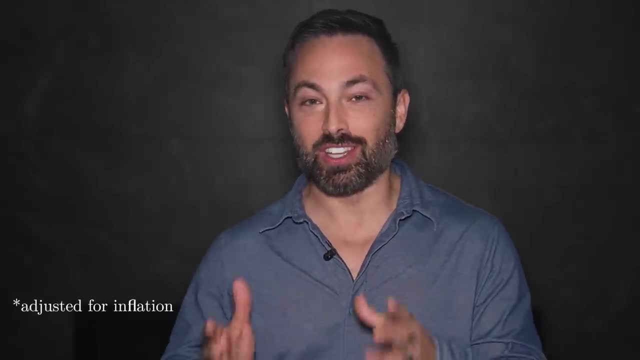 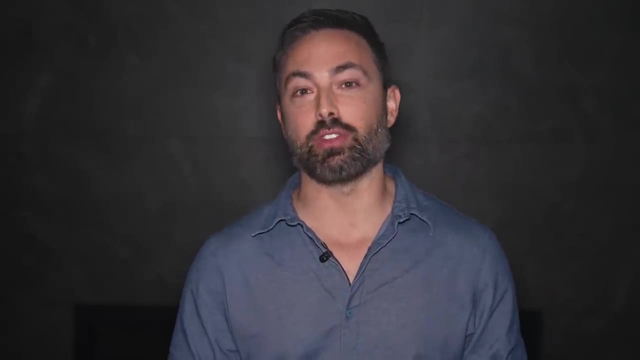 And both countries spent around 10 trillion dollars developing these weapons. Both would have been better off if they had cooperated and agreed not to develop this technology further, But Because they both acted in their own best interest, they ended up in a situation where 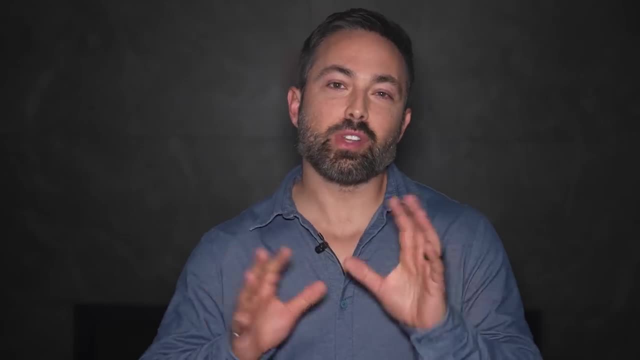 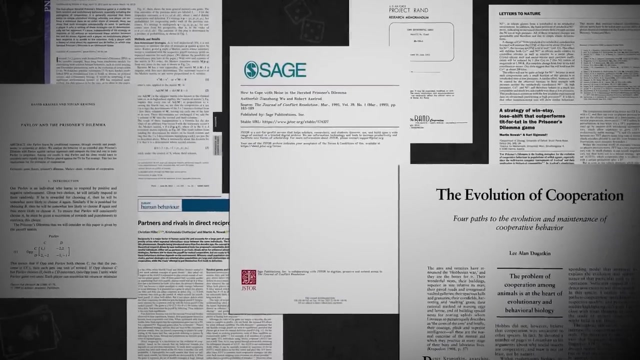 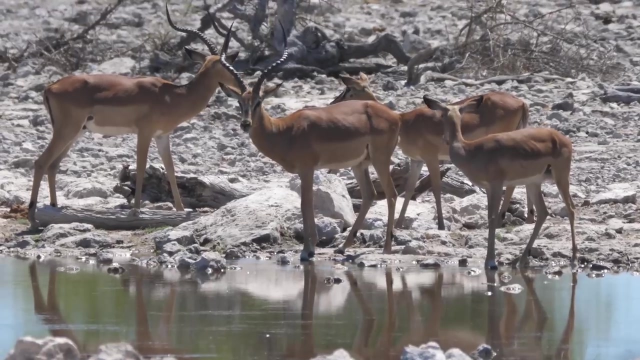 everyone was worse off. The Prisoner's Dilemma is one of the most famous games in game theory. Thousands and thousands of papers have been published on versions of this game. In part that's because it pops up everywhere. Impalas living in between African woodlands and savannas are prone to catching ticks. 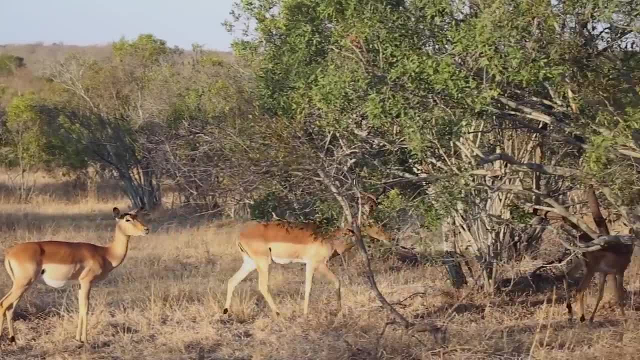 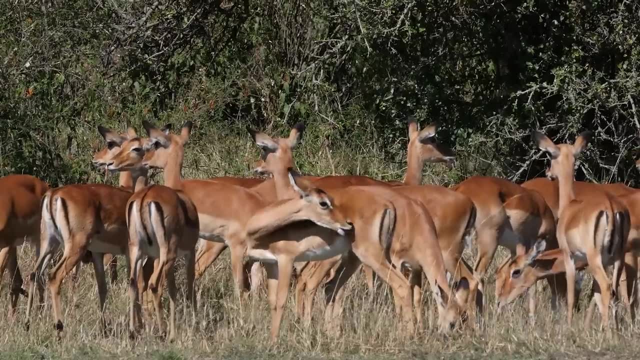 which can lead to infectious diseases, paralysis, even death. So it's important for impalas to remove ticks, and they do this by grooming, But they can't reach all the spots on their bodies and therefore they need another impala to groom them. 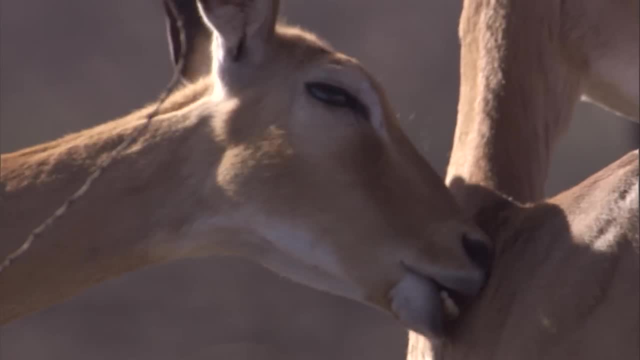 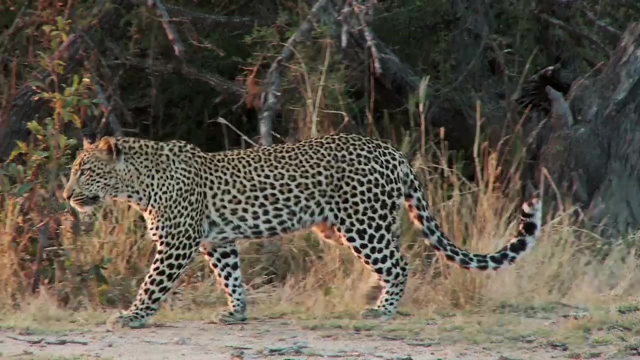 Now, grooming someone else comes at a cost. It costs saliva, electrolytes, time and attention, all vital resources under the hot African sun where a predator could strike at any moment. So for the other impala, it would be best not to pay this cost. 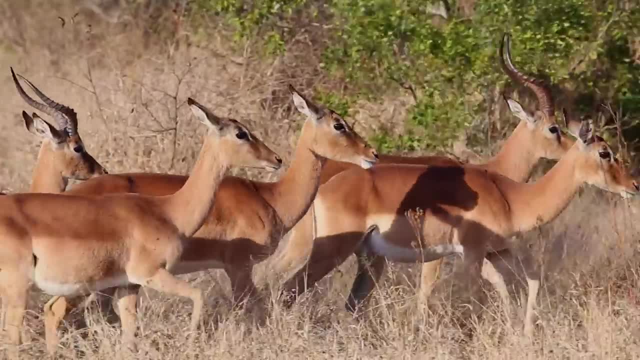 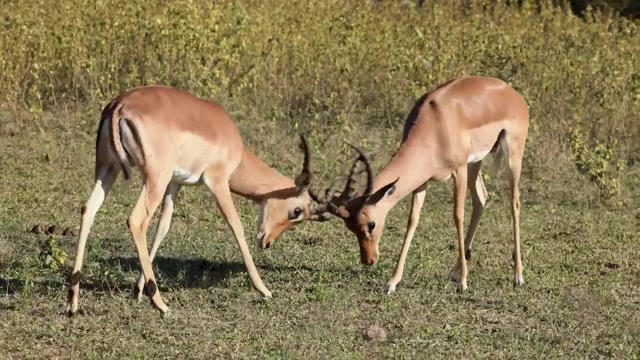 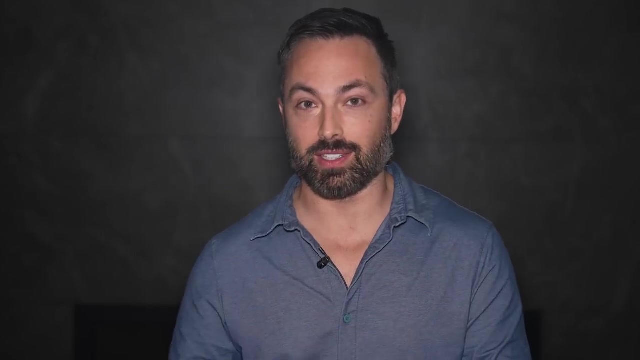 But then again It too. Impalas will need help grooming. So all impalas face a choice: Should they groom each other or not? In other words, should they cooperate or defect? Well, if they only interact once, then the rational solution is always to defect. 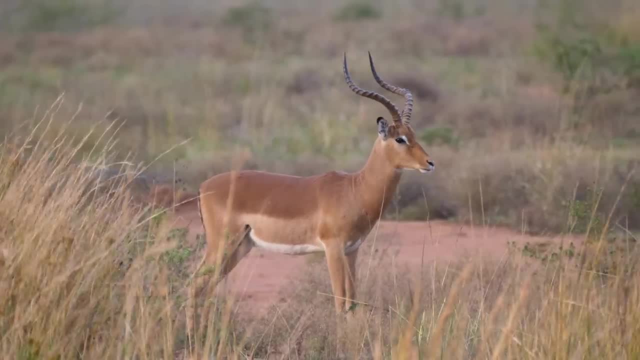 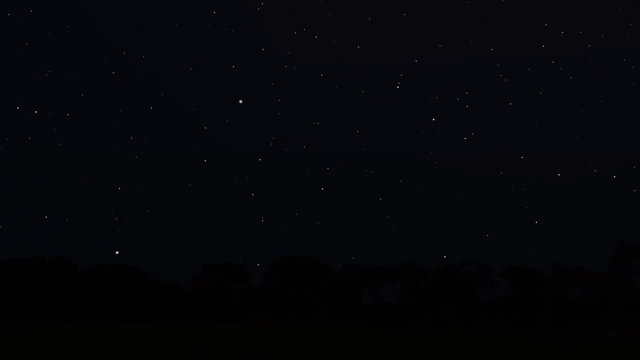 That other impala is never going to help you, so why bother? But the thing about a lot of problems is that they're not a single Prisoner's Dilemma. Impalas see each other, day after day and the same situation keeps happening over and over. 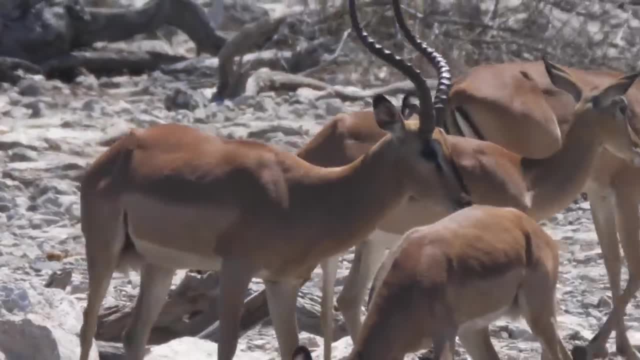 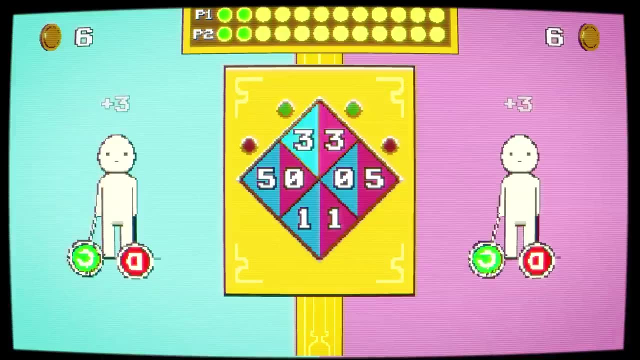 again. So that changes the problem, Because instead of playing the Prisoner's Dilemma just once, you're now playing it many, many times, And if I defect now, then my opponent will know that I defected and they can use that. 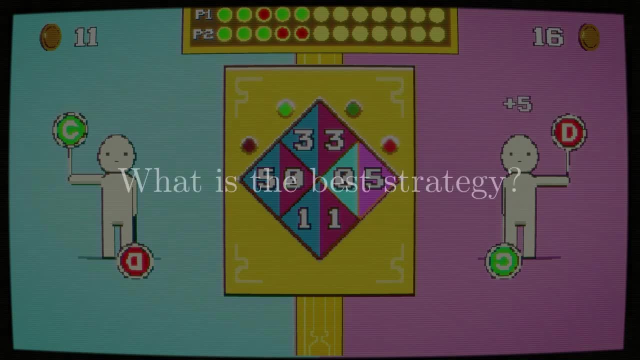 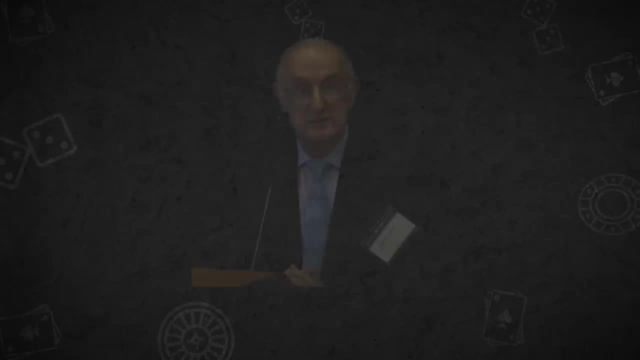 against me in the future. So what is the best strategy in this repeated game? That is what Robert Axelrod, a political scientist, wanted to find out. So in this video, I'm going to talk about the best strategy in this repeated game. 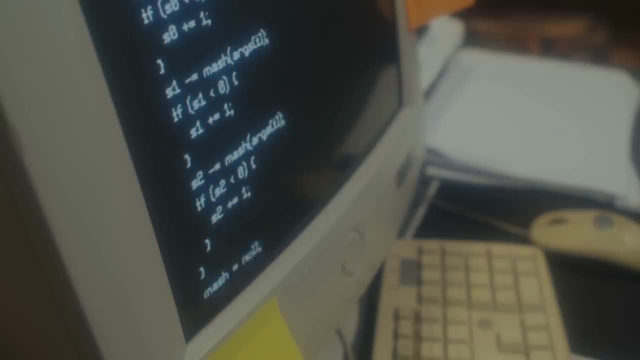 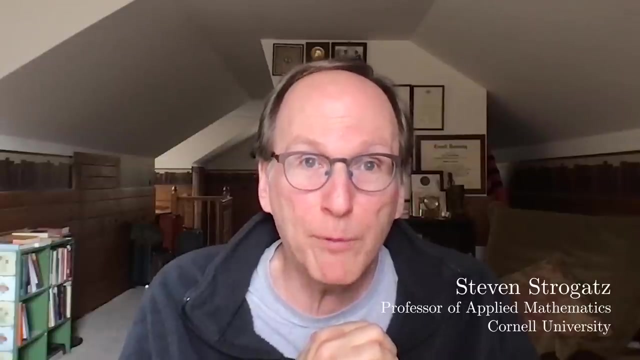 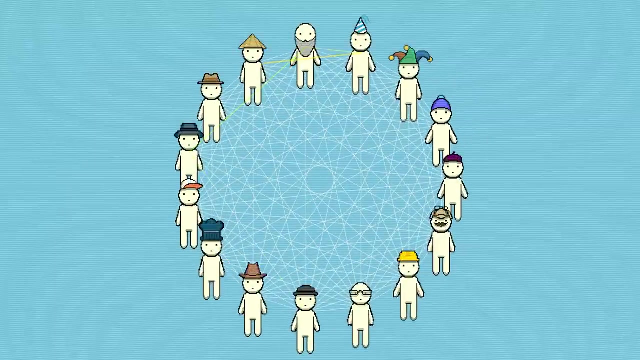 So in 1980, he decided to hold a computer tournament. Axelrod called these programs strategies. Each strategy would face off against every other strategy and against a copy of itself, And each matchup would go for 200 rounds. That's important and we'll come back to it. 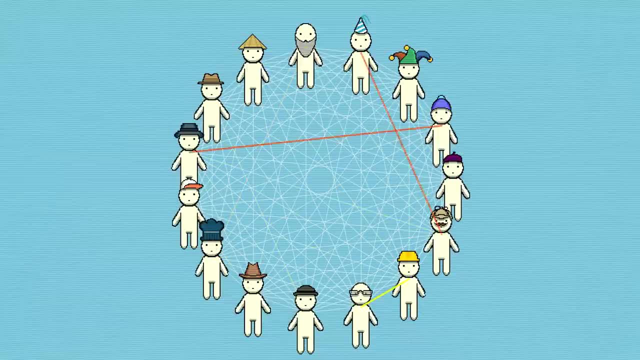 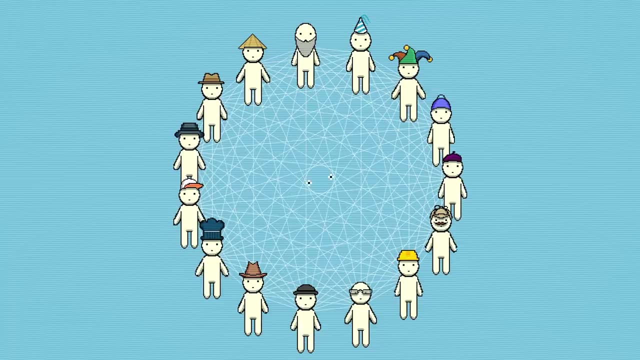 Now, Axelrod used points instead of coins, But the payoffs were the same. The goal of the tournament was to win as many points as possible, And in the end the whole tournament was repeated five times over to ensure the success was robust and not just a fluke. 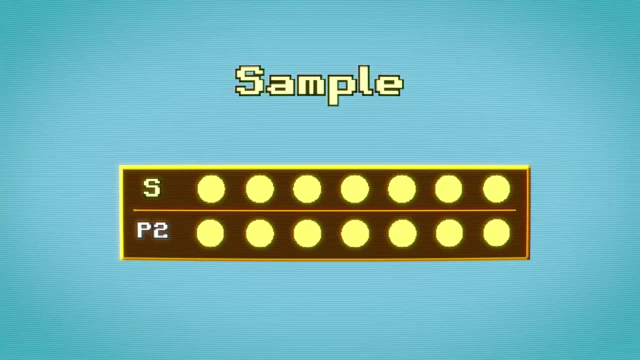 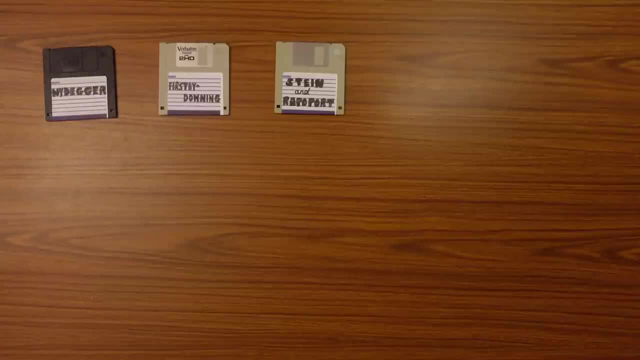 Axelrod gave an example of a simple strategy. It would start each game by cooperating and only defect after its opponent had defected twice in a row. In total, Axelrod received 14 strategies, and he added a 15th called Random, which 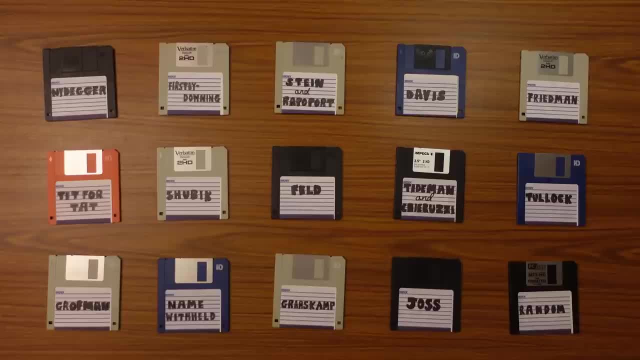 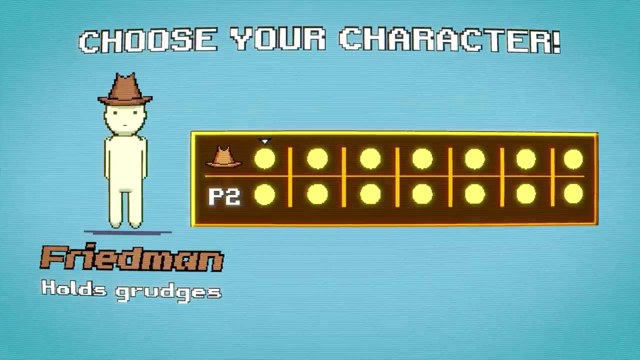 just randomly cooperates or defects 50% of the time. All strategies were loaded onto a single computer where they faced off against each other. One of the strategies was called Freedman. It starts off by cooperating, but if its opponent defects just once, it will keep defecting. 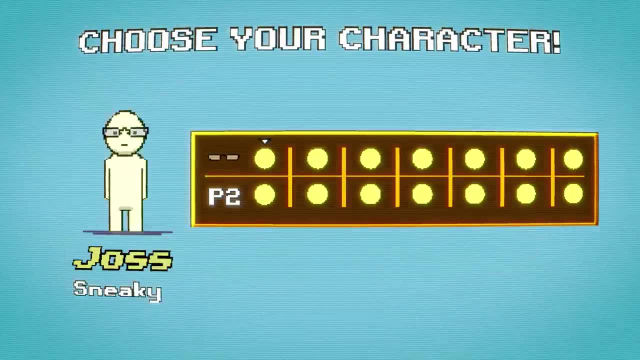 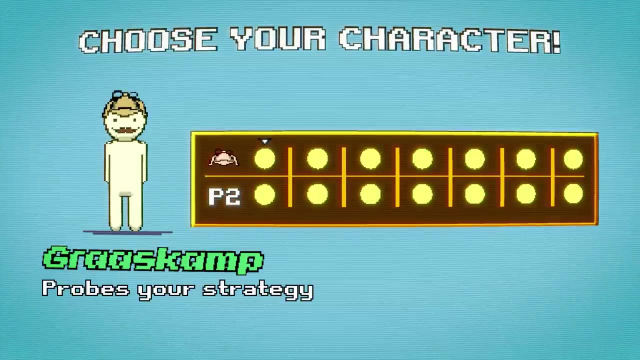 for the remainder of the game. Another strategy was called Joss. It also starts by cooperating, but then it just copies what the other player did on the last move. 50% of the time Joss gets sneaky and defects. There was also a rather elaborate strategy called Grass Camp. 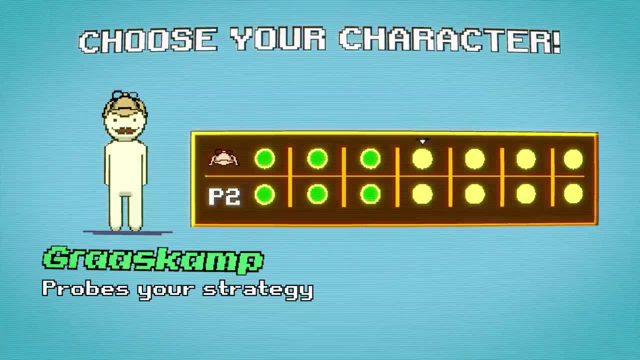 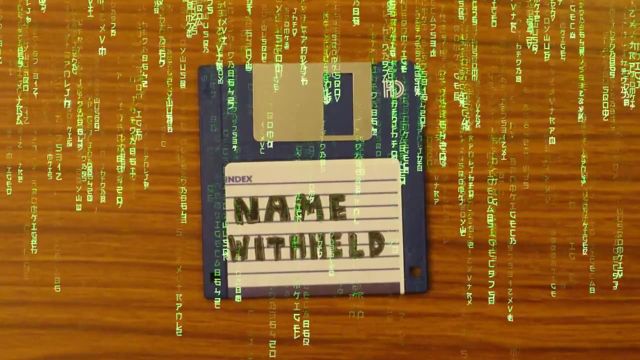 This strategy works the same as Joss, but instead of defecting probabilistically, Grass Camp defects in the 50th round. to try and probe the strategy of its opponent and see if it can take advantage of any weaknesses, The most elaborate strategy was Name Withheld, with 77 lines of code. 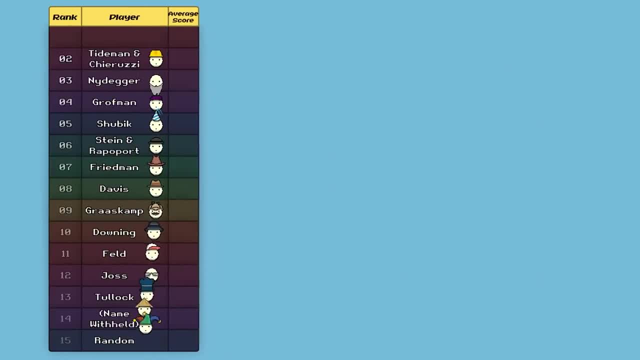 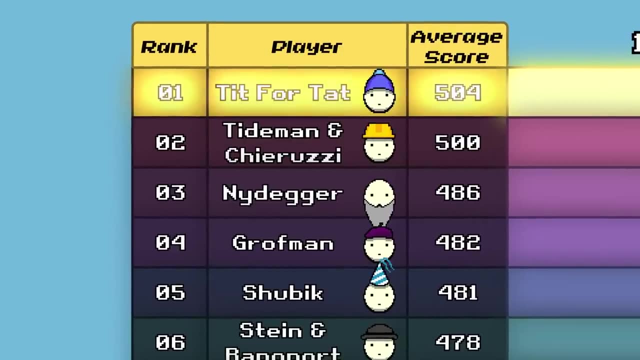 After all, the games were played, the results were tallied up and the leaderboard established. The crazy thing was that the simplest program ended up winning- A program that came to be called Tit for Tat. Tit for Tat starts by cooperating, and then it copies exactly what its opponent did in. 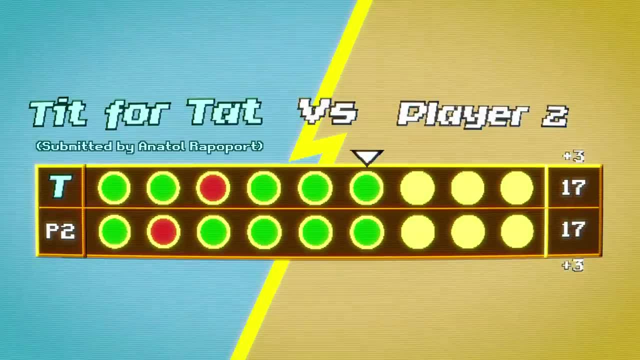 the last move. So it would follow: cooperation with cooperation and defection with defection. But only once. if its opponent goes back to cooperating, so does Tit for Tat. When Tit for Tat played against Freedman, both started by cooperating and they kept. 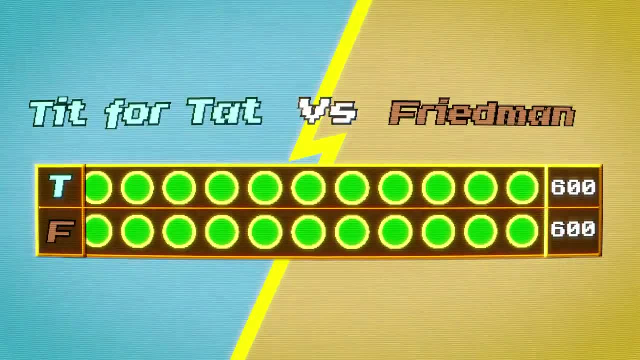 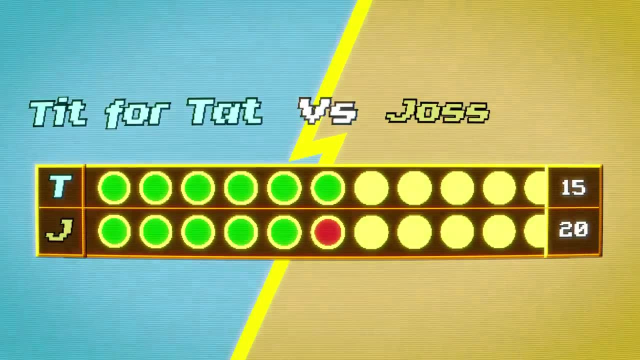 cooperating, Both ending up with perfect scores for complete cooperation. When Tit for Tat played against Joss, they too started by cooperating, but then, on the sixth move, Joss defected. This sparked a series of back and forth defections, a sort of echo effect. 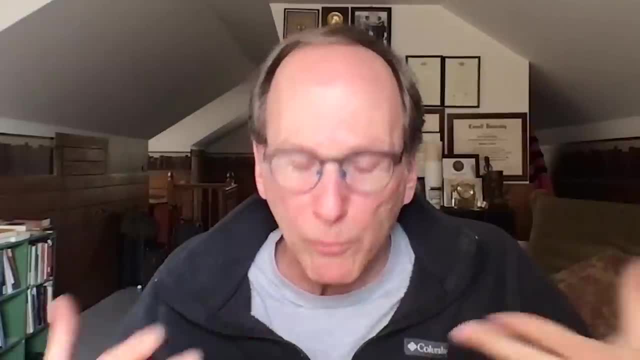 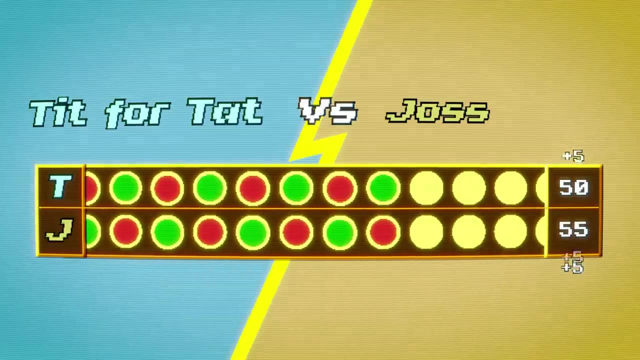 Okay. so now you've got this alternating thing, which will remind you of some of the politics of the world today, where we have to do something to you because of what you did to us, And then when this weird program throws in a second unprovoked defection, now it's really. 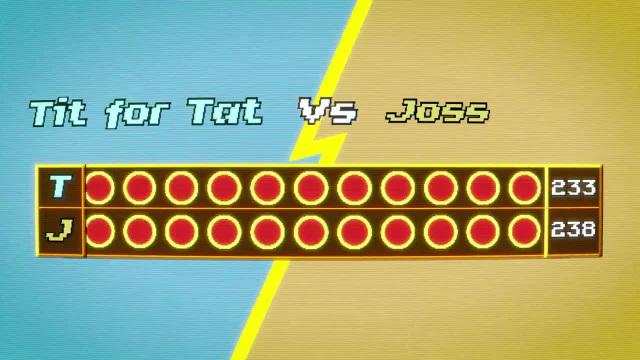 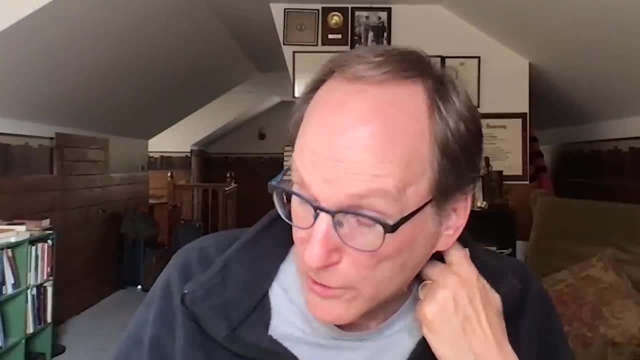 bad, Because now both programs are going to defect on each other for the rest of the game, And that's also like some of the things that we're seeing in politics today and in international relations. As a result of these mutual retaliations, both Tit for Tat and Joss did poorly. 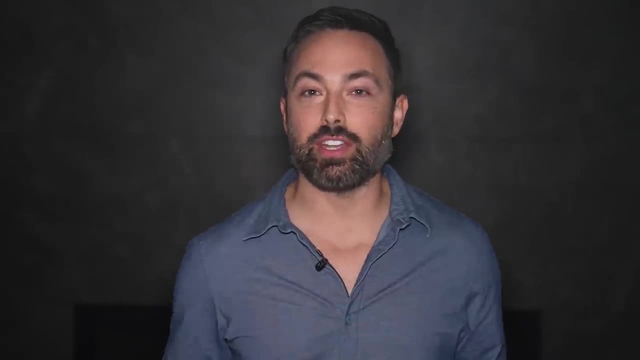 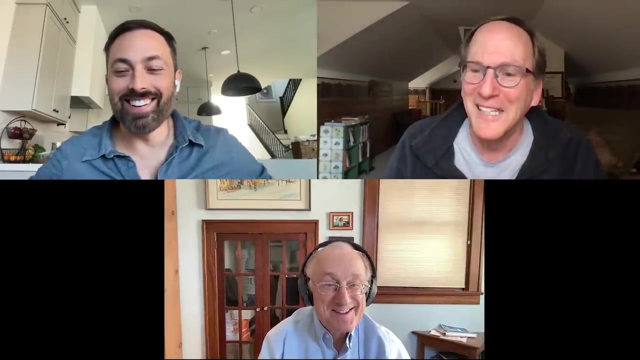 But because Tit for Tat managed to cooperate with enough other strategies, it still won the tournament. Hey, my god, there's Professor Axelrod. Hey, There's Stephen Stewart. Wow, what a treat. I'm so happy. Wow, what a treat this is. 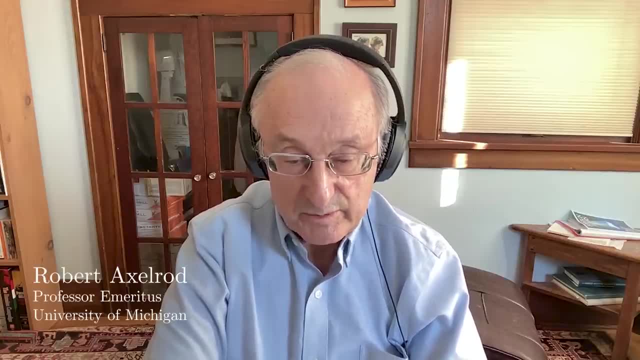 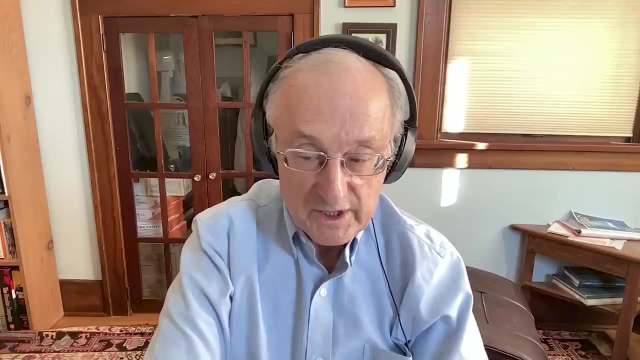 I imagined initially it'd be sort of like computer chess, where you need a pretty complicated program to play a sophisticated game. But in fact it was not like that at all. It was the simplest strategy that did the best. So I analyzed how that happened. 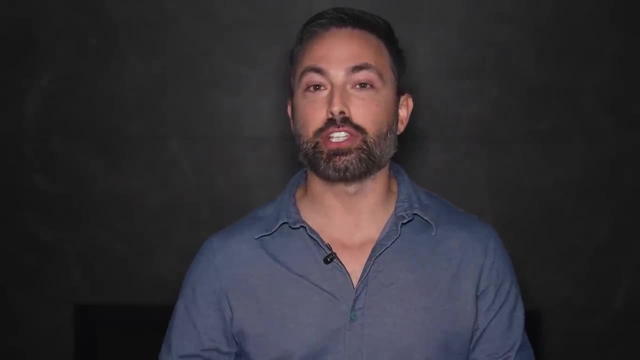 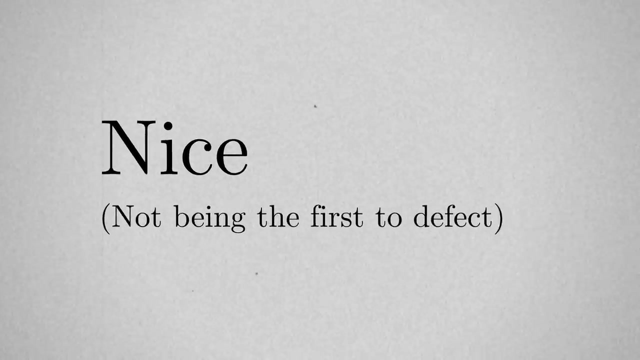 Axelrod found that all the best performing strategies, including Tit for Tat, shared four qualities. First, they were all nice, Which just means they are not the first to defect. So Tit for Tat is a nice strategy. It can defect, but only in retaliation. The opposite of nice is nasty. That's a strategy that defects first. So Joss is nasty. Out of the fifteen strategies in the tournament, eight were nice and seven nasty. The top eight strategies were all nice And even the worst performing nice strategy still far outscored the best performing nasty. 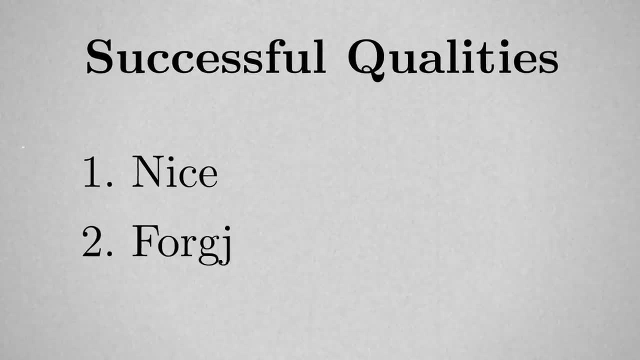 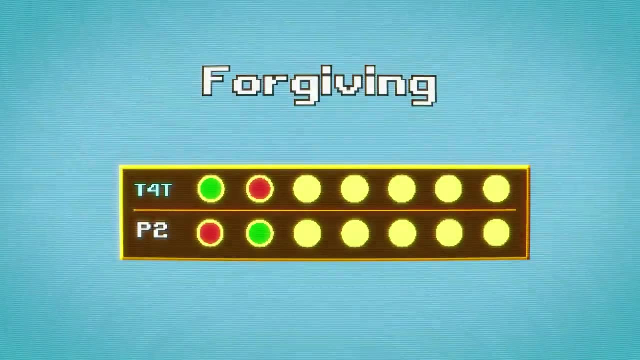 one. The second important quality was being forgiving. A forgiving strategy is one that can retaliate but it doesn't hold a grudge. So Tit for Tat is a forgiving strategy. It retaliates when its opponent defects, but it doesn't let defections from before the 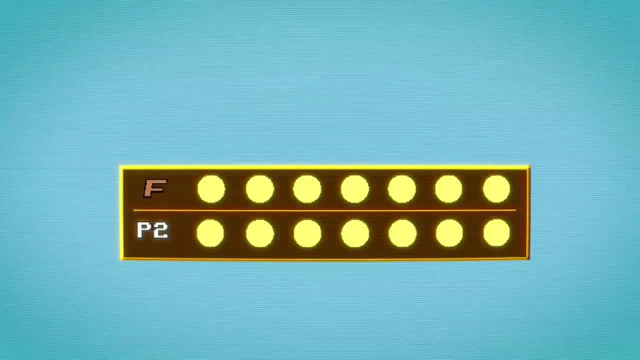 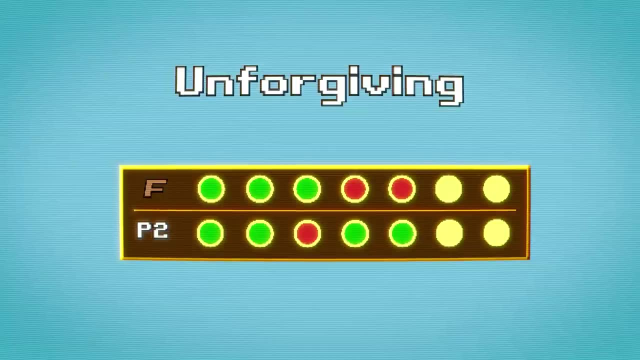 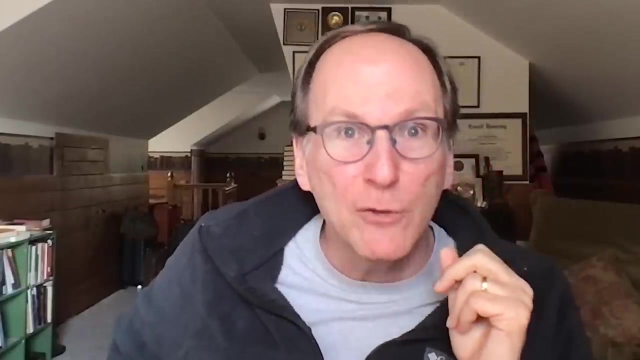 last round influence its current decisions. Friedman, on the other hand, is maximally unforgiving. After the first, defection just from the opponent would defect for the rest of the game. Okay, that's it, No mercy, And that might feel good to do. 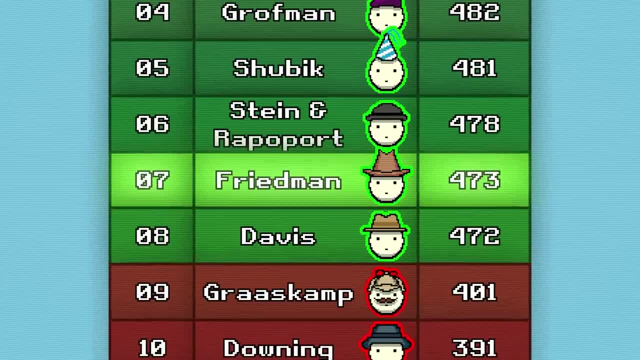 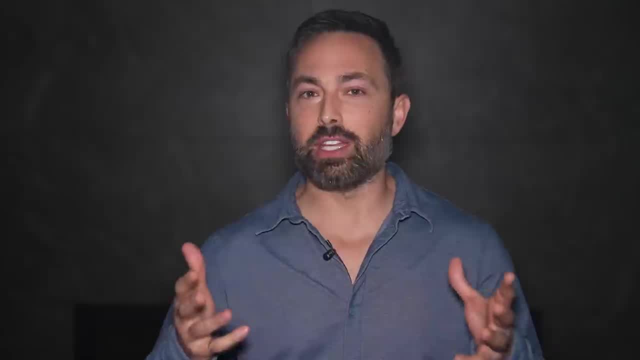 But it doesn't end up working out well in the long run. This conclusion that it pays to be nice and forgiving came as a shock to the experts. Many had tried to be tricky and create subtle, nasty strategies to beat their opponent, and 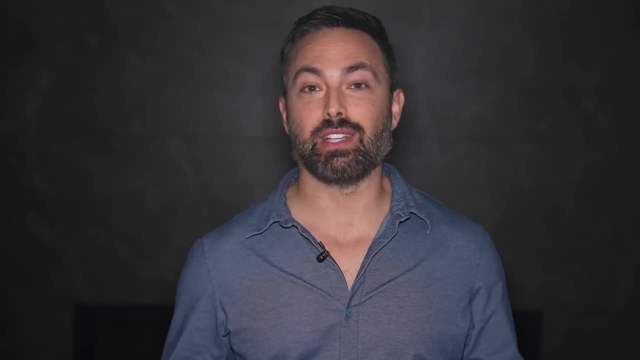 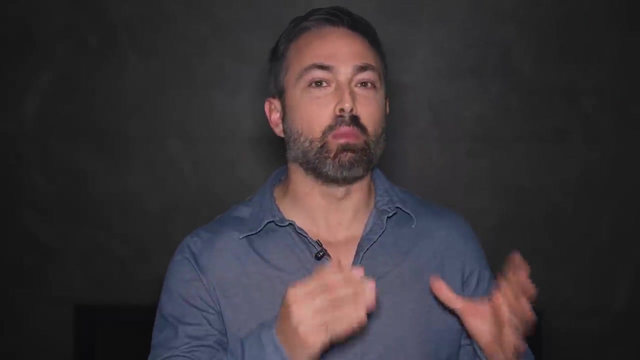 eke out an advantage, But they all failed Instead. in this tournament, nice guys finished first. Now Tit for Tat is quite forgiving, but it's possible to be even more forgiving. Axelrod's sample strategy only defects after its opponent defected twice in a row. 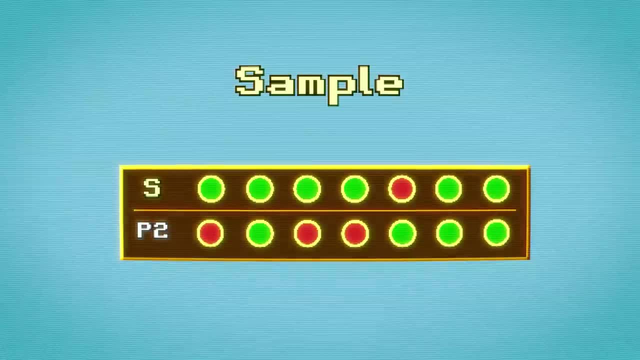 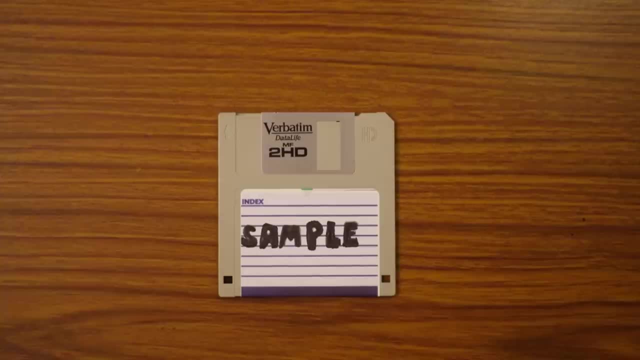 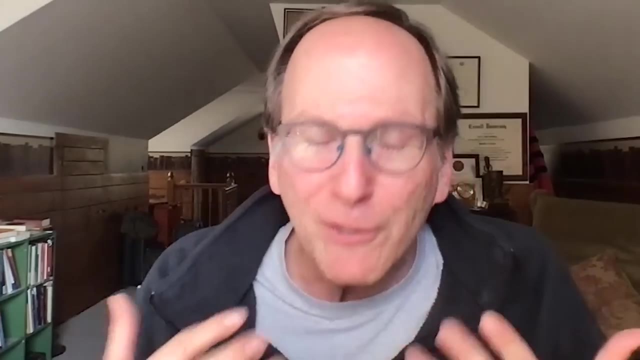 That's a good thing. It was Tit for Two Tats. Now that might sound overly generous, but when Axelrod ran the numbers he found that if anyone had submitted the sample strategy they would have won the tournament. I mean, it's so clever. 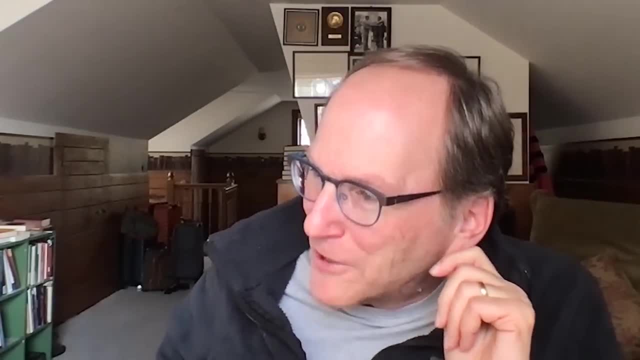 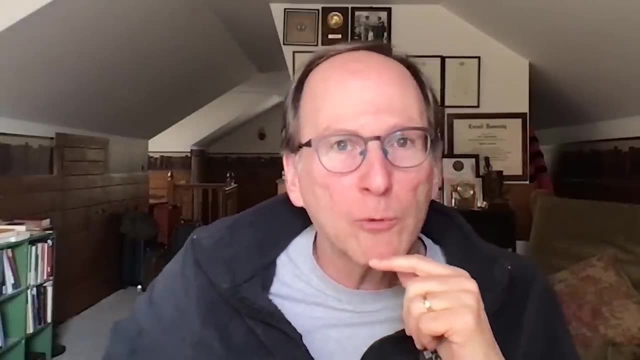 There's so many layers to this story. After Axelrod published his analysis of what happened, or circulated it among these game theorists, he said: now that we all know what worked. well, uh, I don't know. Let's try again. 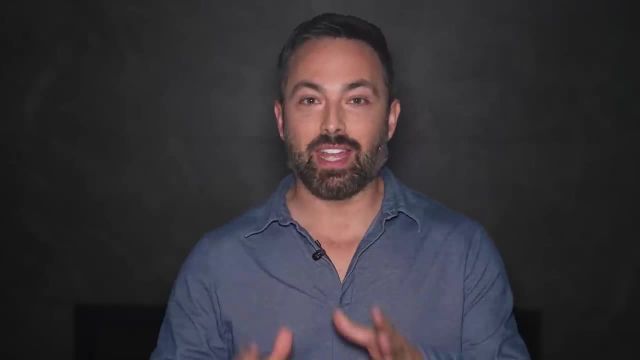 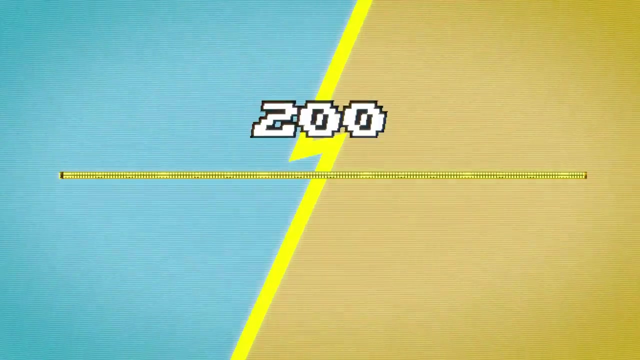 So he announced a second tournament where everything would be the same, except for one change: the number of rounds per game. See, in the first tournament each game lasted precisely 200 rounds, And that is important, because if you know when the last round is, then there's no reason. 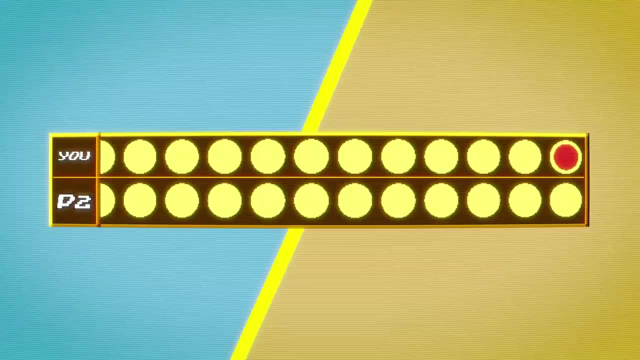 to cooperate in that round, so you're better off defecting. Of course your opponent should reason the same, and so they should also defect in the last round. But if you both anticipate defecting, you're going to lose. You're going to lose. 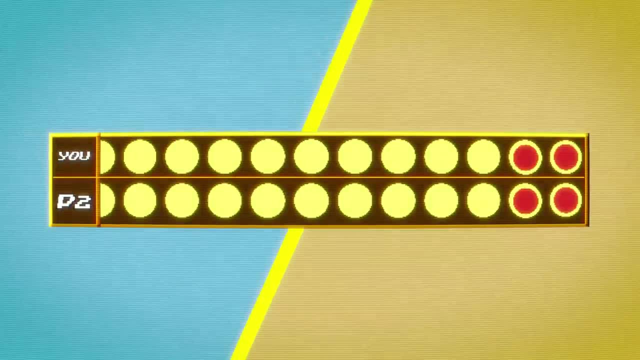 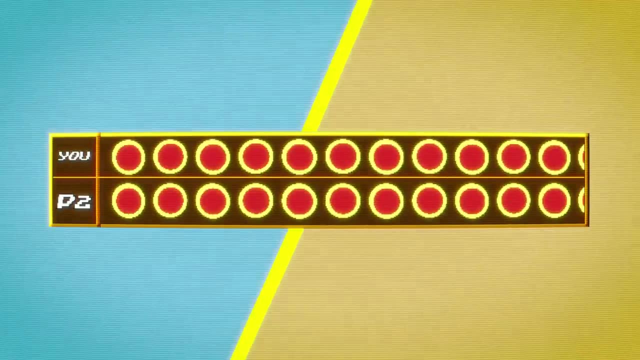 If you anticipate defection in the last round, then there's no reason for you to cooperate in the second to last round or the round before that or before that and so on, all the way to the very first round. And so in Axelrod's tournament it was a very important thing that the players didn't know. 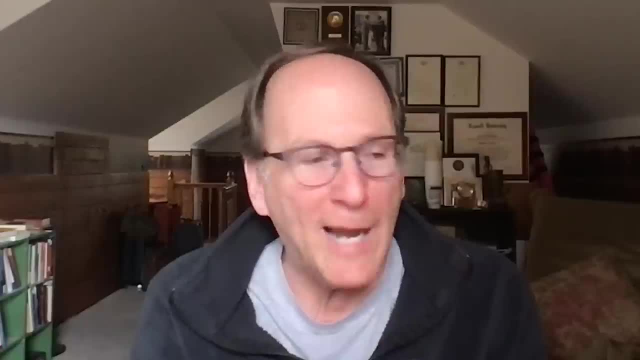 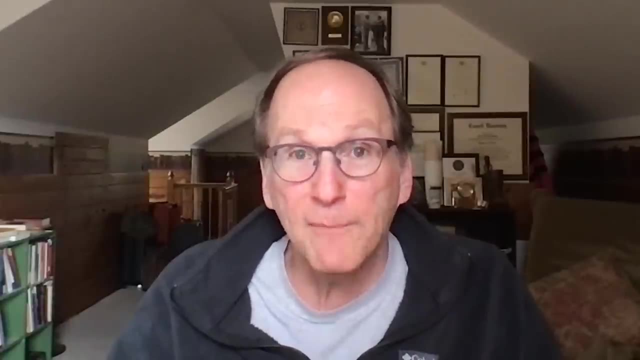 exactly how long they were going to be playing. They knew on average it would be 200 rounds, but there was a random number generator that prevented them from knowing with certainty. Yeah, if you're not sure when it ends, then you have to kind of keep cooperating, because 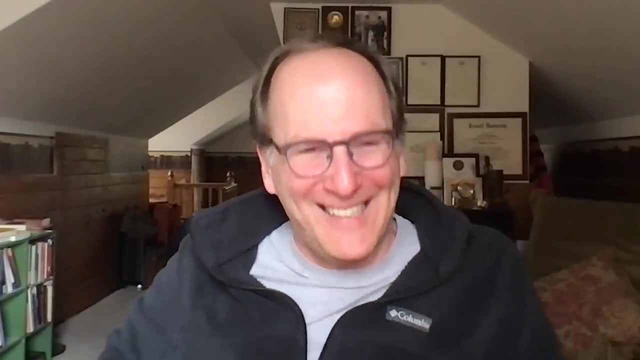 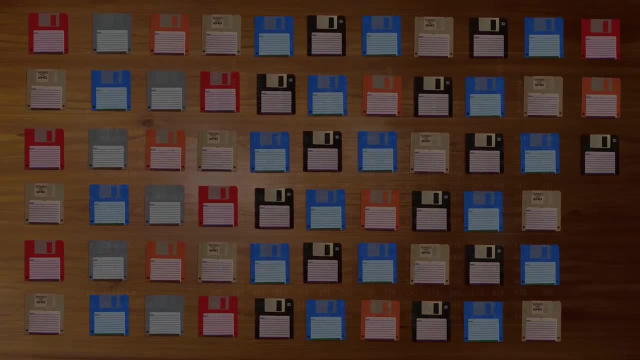 you might keep going and you might need them on your side. For this second tournament, Axelrod received 62 entries and again added random. The contestants had gotten the results and analysis from the first tournament and could use this information to their advantage. 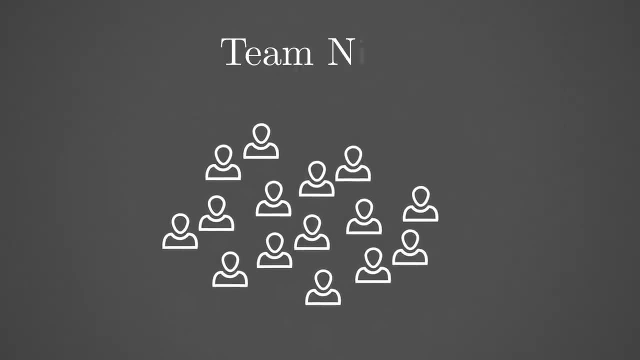 This created two camps. Some thought that clearly, being nice and forgiving were winning qualities, so they submitted nice and forgiving strategies. One even submitted tit for two tats. The second camp: They anticipated that others would be nice and extra forgiving and therefore they submitted. 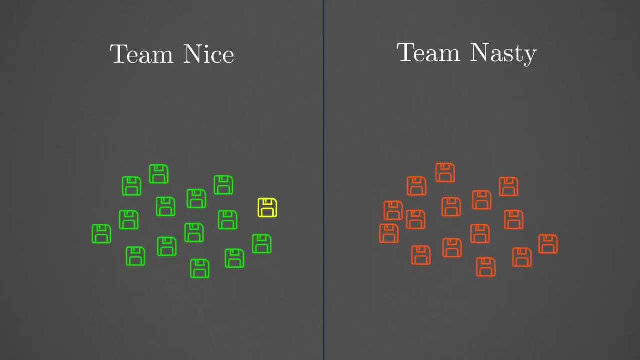 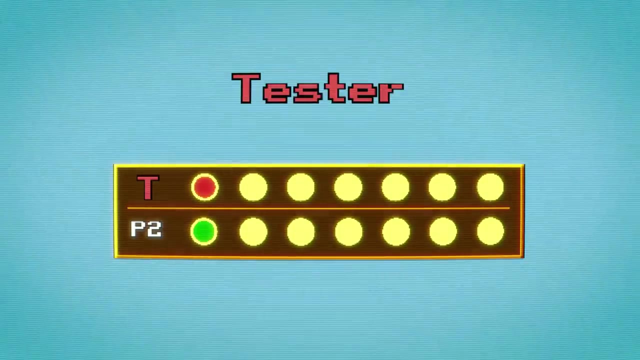 nasty strategies to try to take advantage of those that were extra forgiving. One such strategy was called Tester. It would defect on the first move to see how its opponent reacted. If it retaliated, Tester would apologize and play tit for tat for the remainder of the 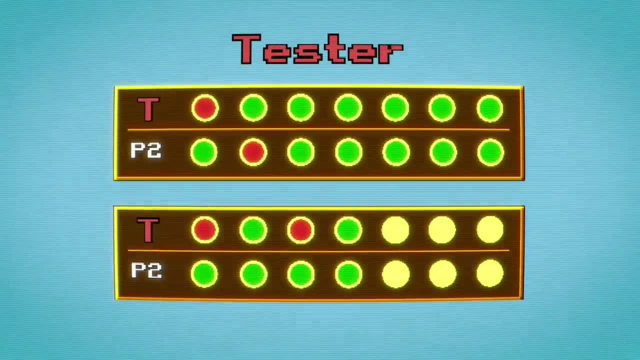 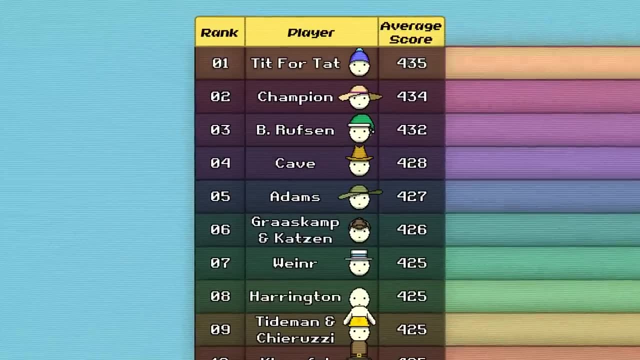 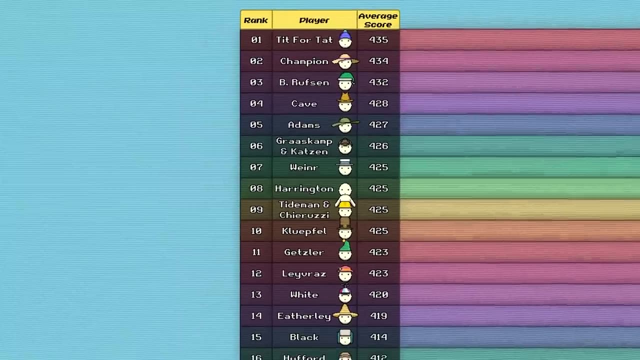 game. If it didn't retaliate, Tester would defect every other move after that. But again, being nasty didn't pay And once again tit for tat was the most effective. Nice strategies again did much better In the top 15, only one was not nice. 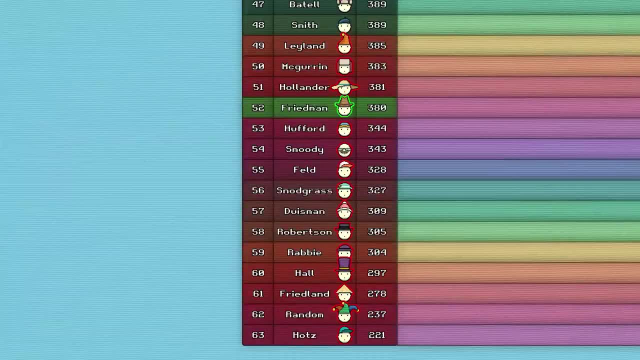 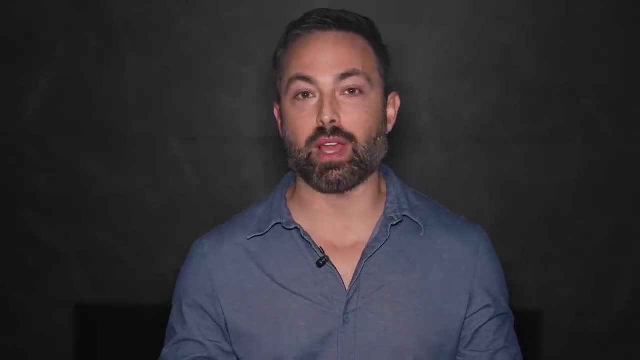 Similarly in the bottom 15, only one was not nasty. After the second tournament, Axelrod identified the other qualities that distinguish the better-performing strategies. The third is being retaliatory, which means if your opponent defects, strike back immediately. 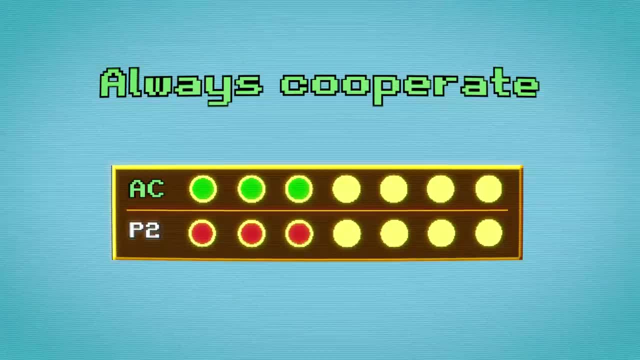 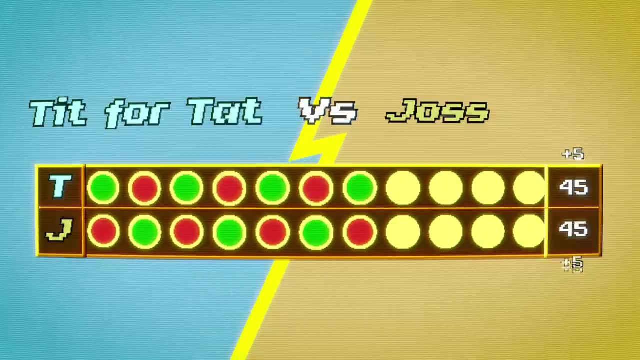 Don't be a pushover. Don't be a pushover. Always cooperate is a total pushover, and so it's very easy to take advantage of Tit, for tat, on the other hand, is very hard to take advantage of. The last quality that Axelrod identified is being clear. 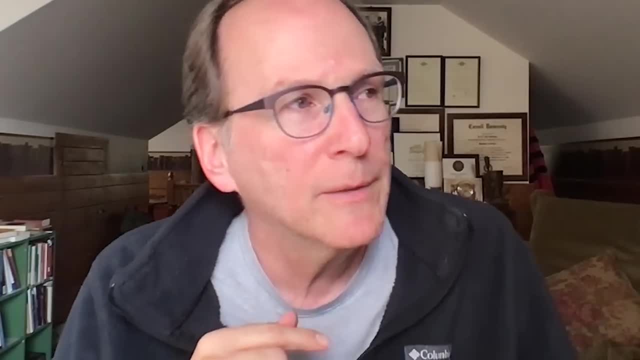 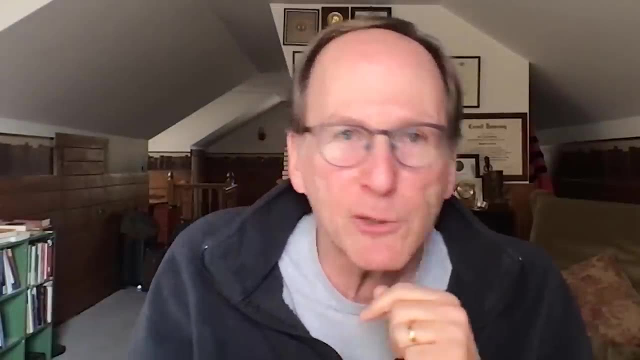 Programs that were too opaque, that were too similar to a random program. you couldn't figure them out because they were so complicated. it was very hard to establish any pattern of trust with a program like that because you couldn't figure out what it was doing. 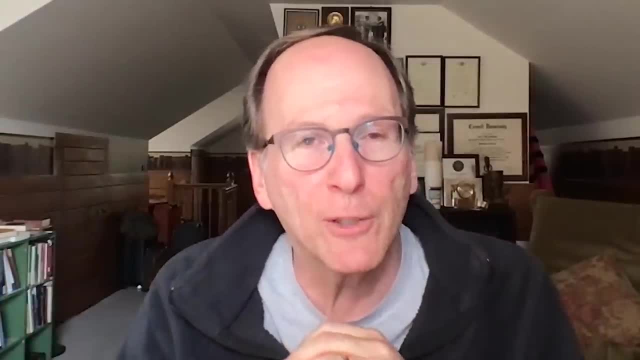 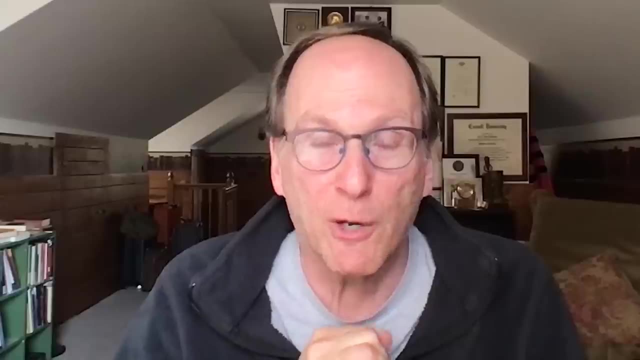 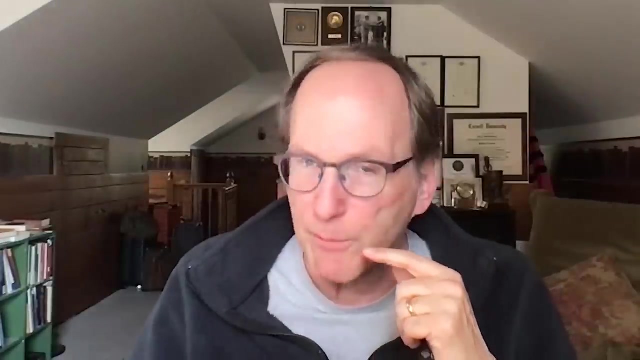 I mean the other programs it was playing- couldn't figure them out, and so they would end up more or less defaulting to thinking every turn is like the last time I'm going to see you, so I might as well defect. What to me is mind-blowing about this is that these four principles, being nice, forgiving, 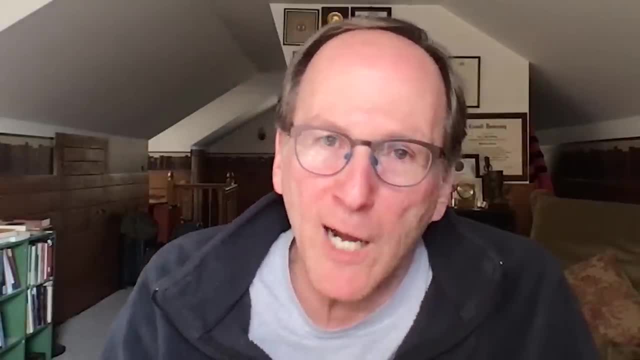 provokable and clear is a lot like the morality that has evolved around the world that is often summarized as an eye for an eye. I mean, it's a lot like the morality that has evolved around the world that is often summarized as an eye for an eye. 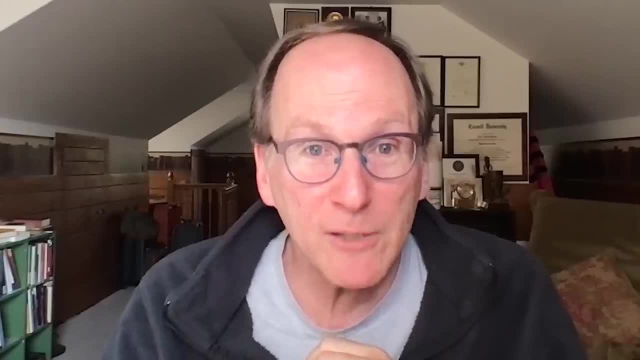 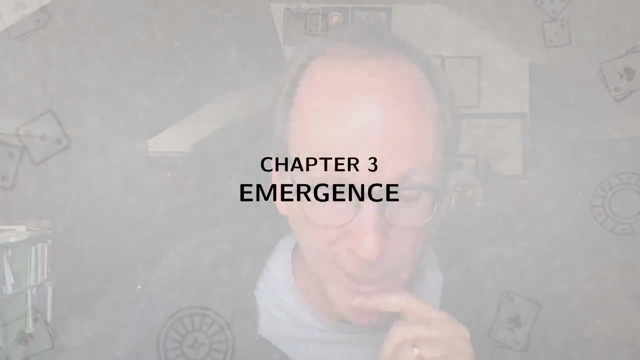 I mean, it's a lot like the morality that has evolved around the world that is often summarized as an eye for an eye. It's not Christianity, by the way. It's not turn-the-other-cheek philosophy, It's some older philosophy. 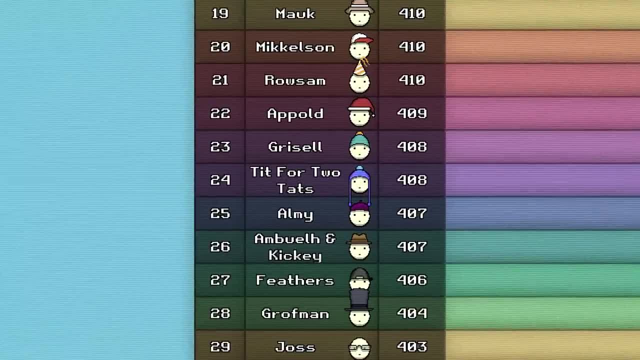 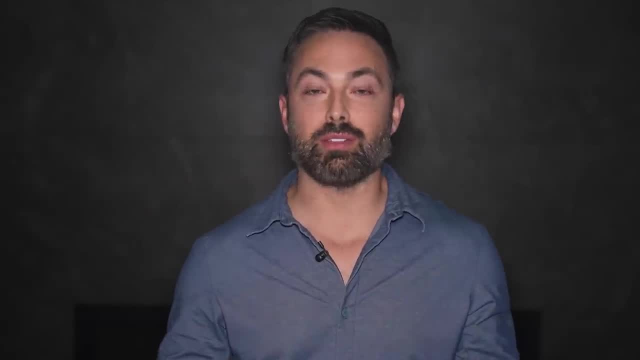 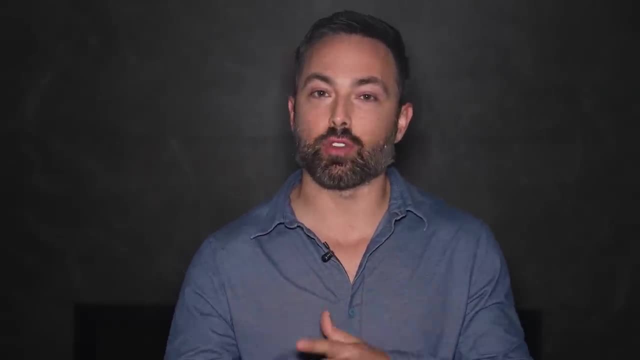 What's interesting is that while Tit-for-Two-Tats would have won the first tournament, it only came 24th in the second tournament. This highlights an important fact In the repeated prisoner's dilemma: there is no single best strategy. The strategy that performs best always depends on the other strategies it's interacting with. 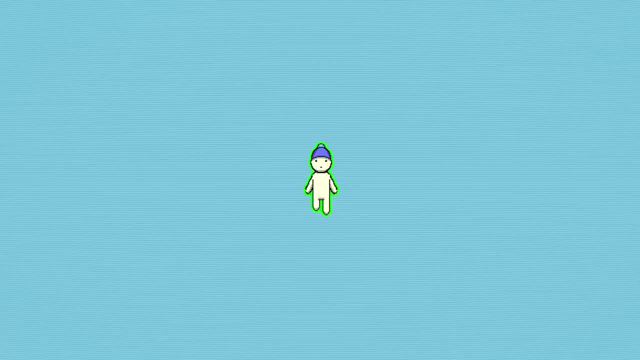 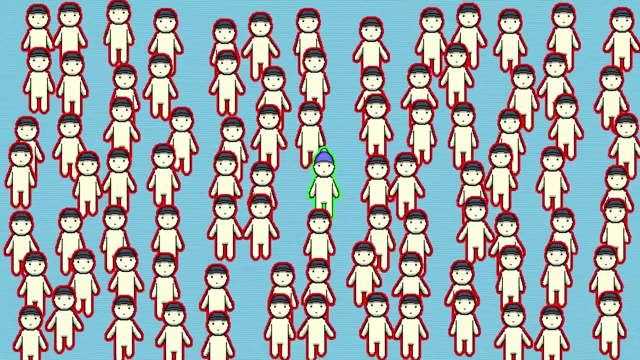 The strategy that performs best always depends on the other strategies it's interacting with. For example, if you put Tit-for-Tat in an environment with only the ultimate bullies of always-defect, then Tit-for-Tat comes in last. I wanted to see whether, for example, the Tit-for-Tat did well, because it did well with 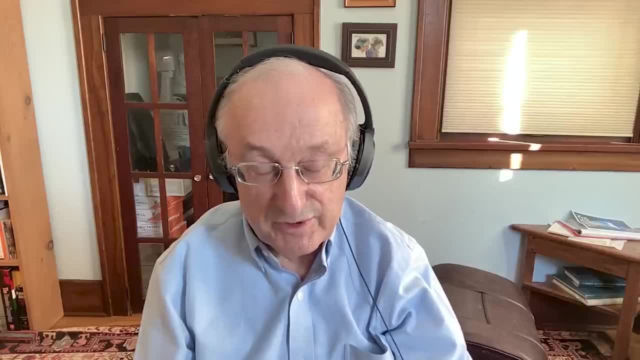 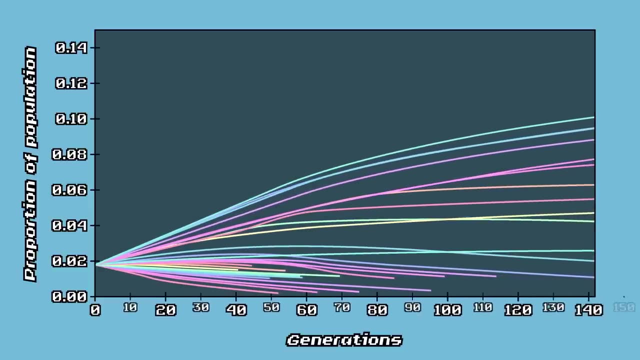 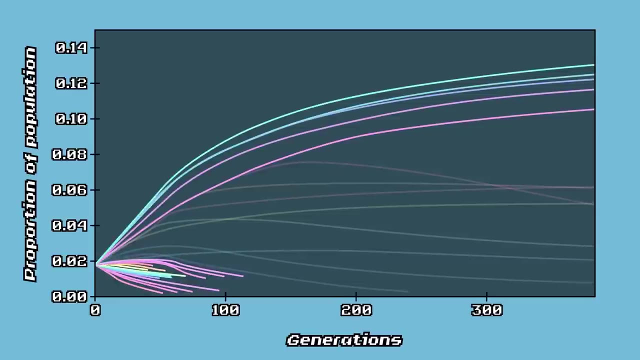 really stupid rules that didn't do well at all themselves, that basically took advantage of people. So he ran a simulation where successful strategies in one generation would see their numbers grow and unsuccessful ones would see their numbers drop. In this simulation, the worst-performing strategies quickly shrink and go extinct while the 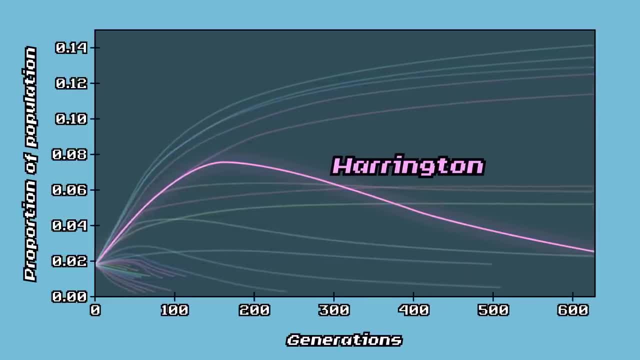 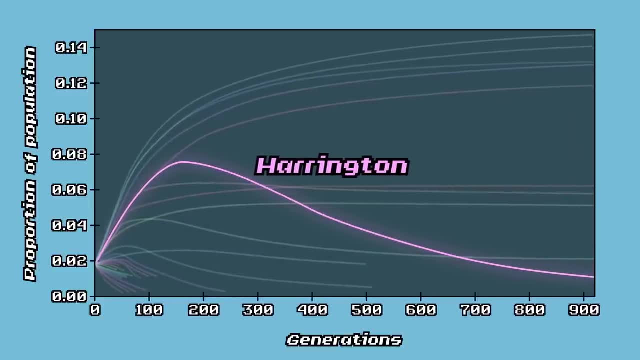 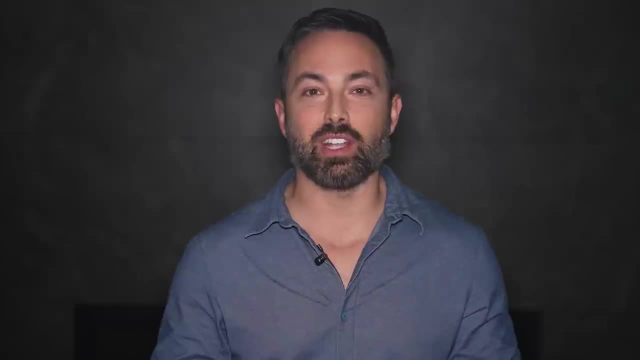 top-performing strategies become more common. Harrington, the only nasty strategy in the top 15, first grew quickly, But then, as the strategies it was preying on went extinct, Harrington's numbers also quickly dropped. This shows a main benefit of this simulation, because it tests how well a strategy does. 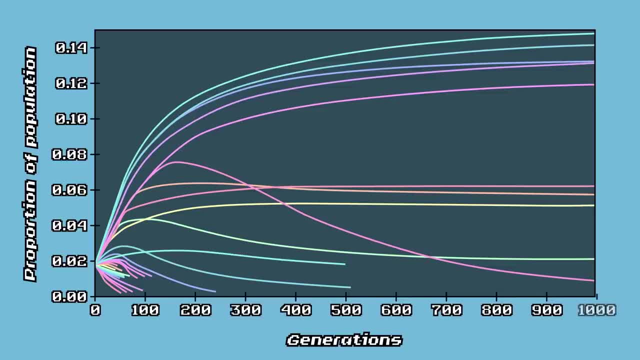 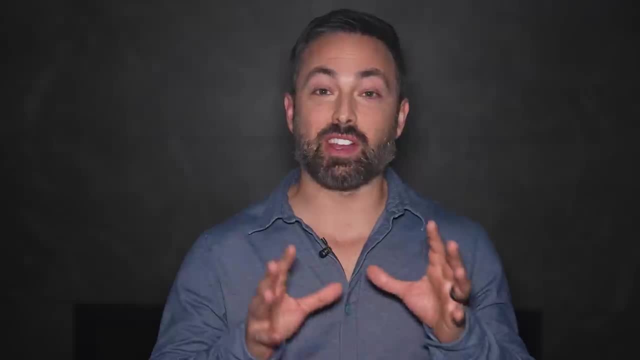 with other successful strategies After a thousand generations. Yeah, Portions are mostly stable and only nice strategies survive. Again, Tit-for-Tat comes out on top, representing 14.5% of the total population. Now this process may sound similar to evolution, but there is a subtle difference, which is: 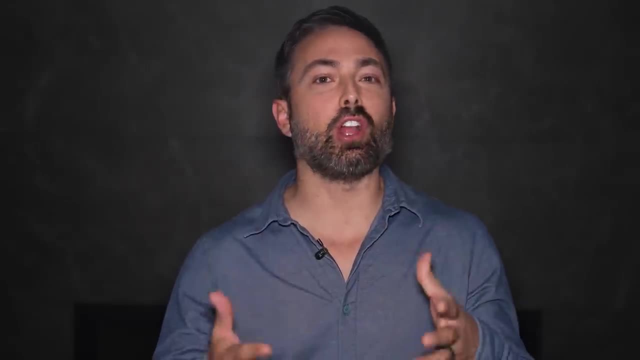 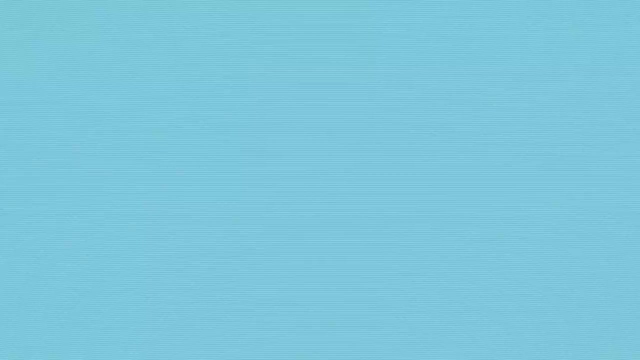 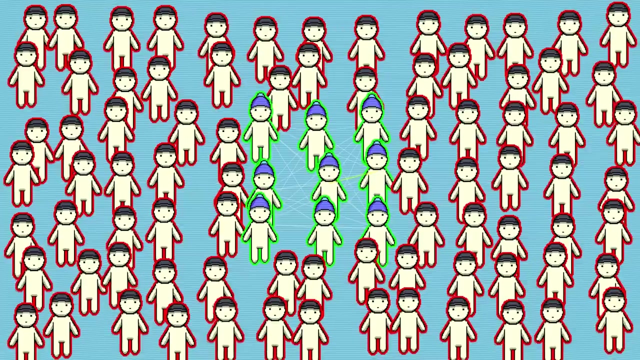 that in this case there are no mutations, so it's actually an ecological simulation. But what if the world you started in was different? Imagine a world that is a really nasty place to live, more or less populated with players that always defect, except there's a little cluster of Tit-for-Tat players that live in. 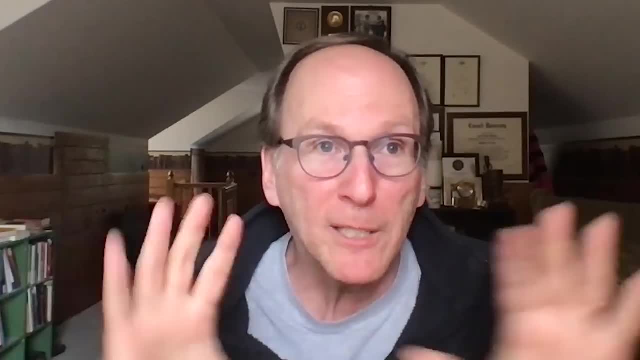 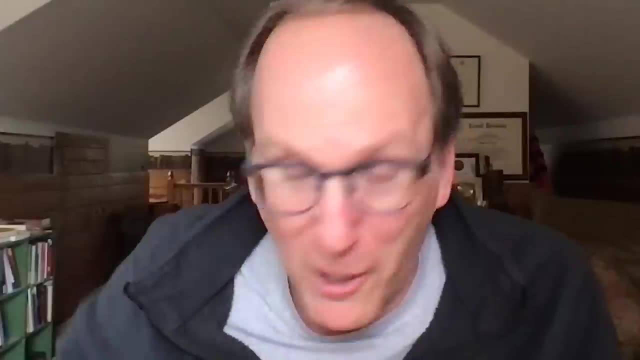 some kind of nucleus And they get to play with each other a lot. because they're geographically sequestered, They will start building up a lot of points and also, because that translates into offspring, they'll start to take over the population. 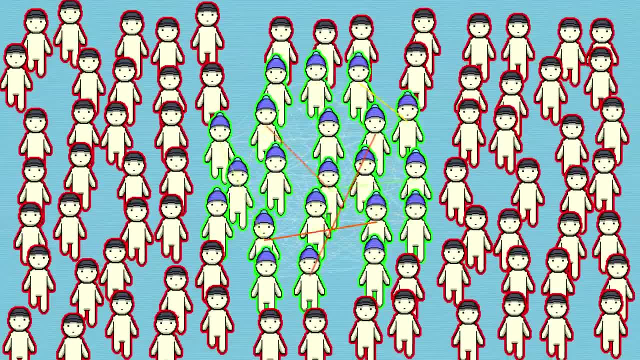 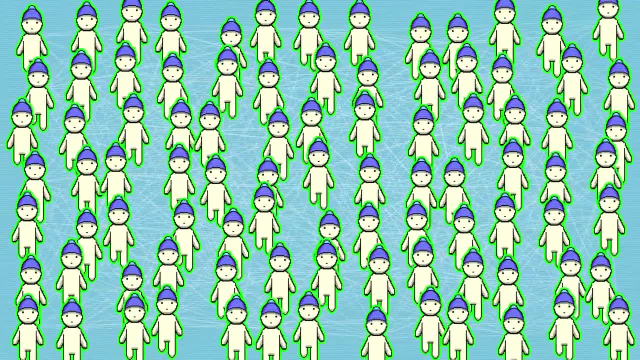 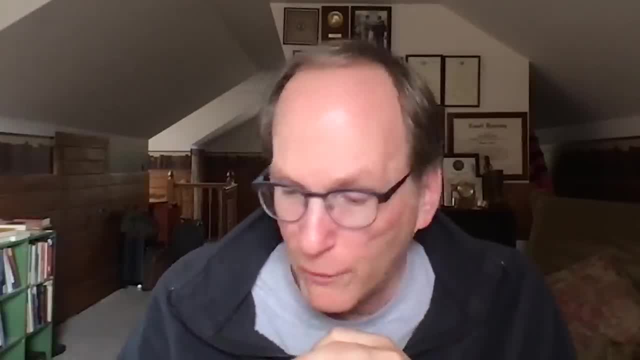 So, in fact, Axelrod showed that a little island of cooperation can emerge and spread and eventually will take over the world, which is fantastic. Yeah, How can cooperation emerge in a population of players who are self-interested, who are not trying to be good because they're good-hearted? 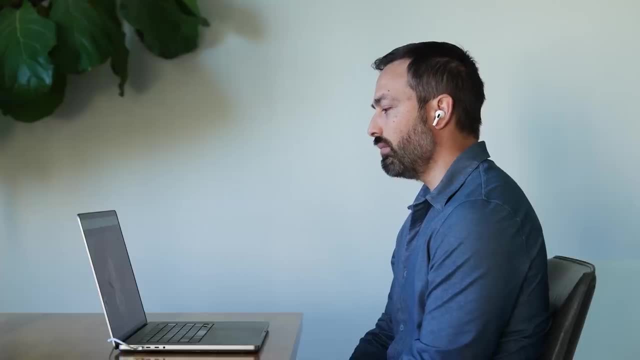 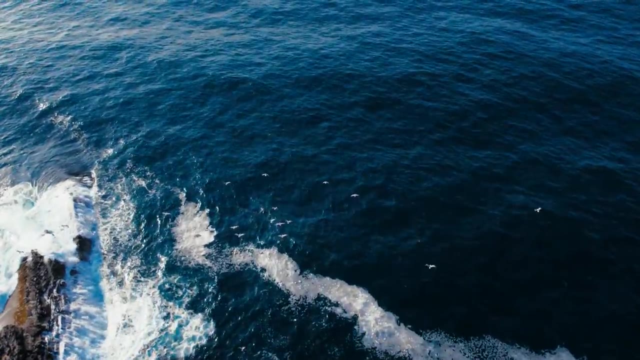 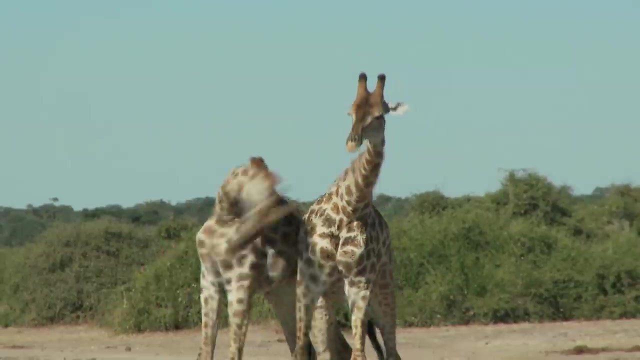 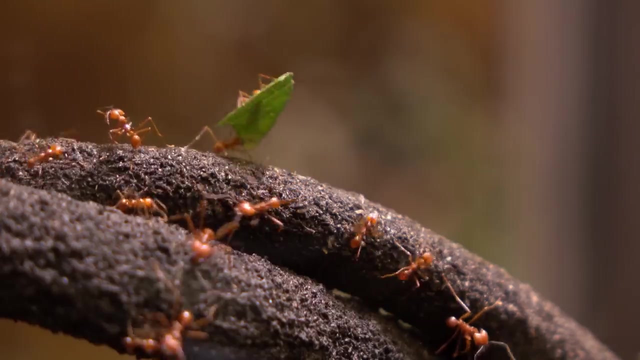 You don't have to be altruistic. You could be looking out for number one for yourself and your own interests, and yet cooperation can still emerge. Some argue that this could explain how we went from a world full of completely selfish organisms… where every organism only cared about themselves, to one where cooperation emerged and flourished. 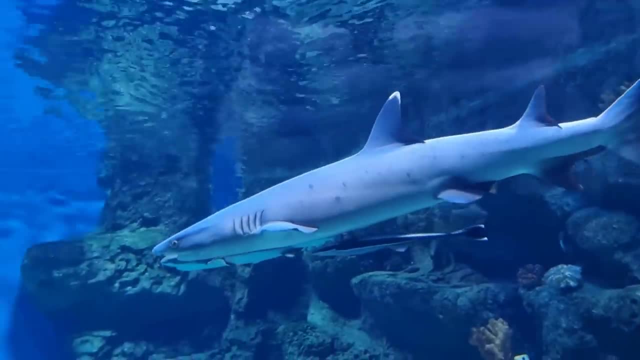 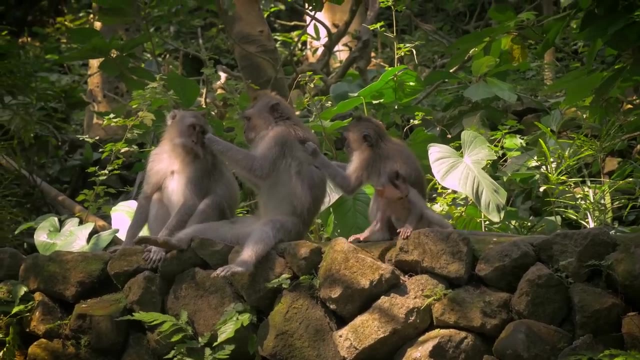 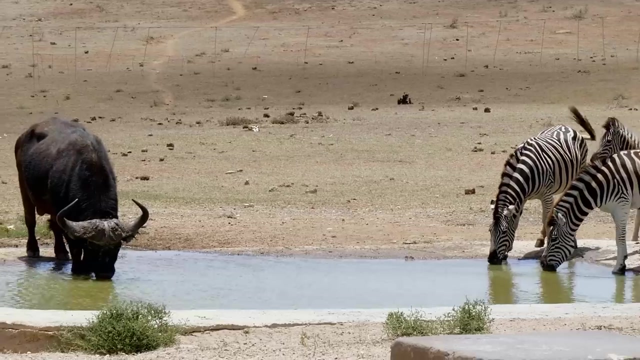 From impalas grooming each other to fish cleaning sharks. Many lifeforms experience conflicts similar to the Prisoner's Dilemma, but because they don't interact just once, both can be better off by cooperating. And this doesn't require trust or conscious thought either, because the strategy could 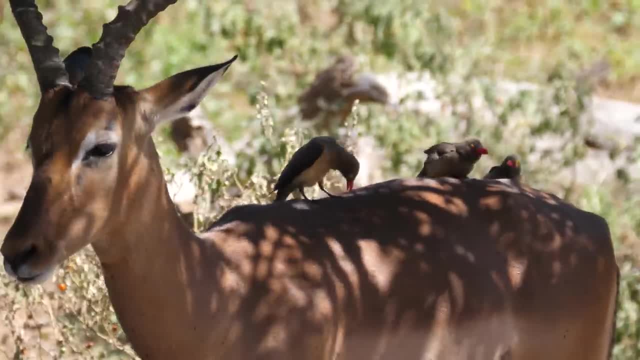 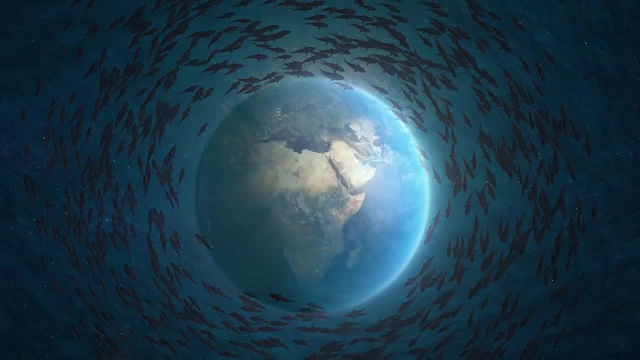 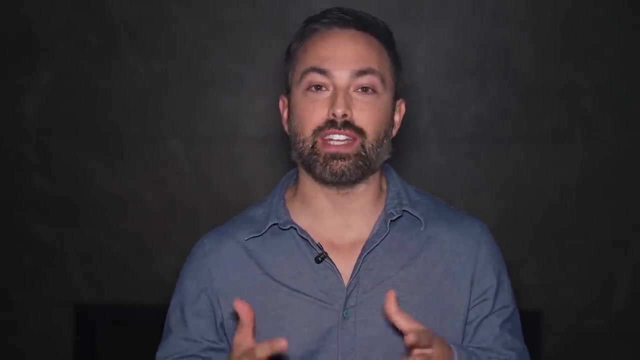 be encoded in DNA, As long as it performs better than the other strategies, it can take over a population. Axelrod's insights were applied to areas like evolutionary biology and international conflicts, But there was one aspect that his original tournaments didn't cover. 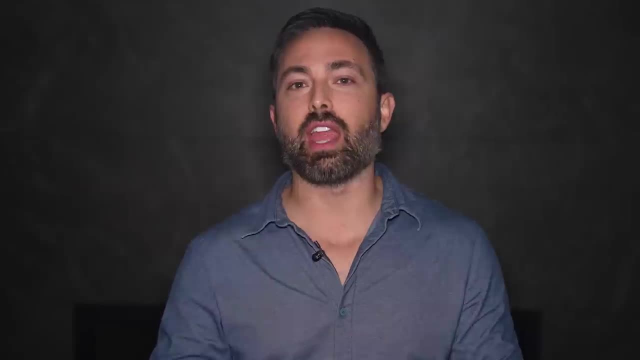 What happens if there is a little bit of random error in the game, Some noise in the system, For example, one player tries to cooperate but it comes across as a defection. Little errors like this happen in the real world all the time. 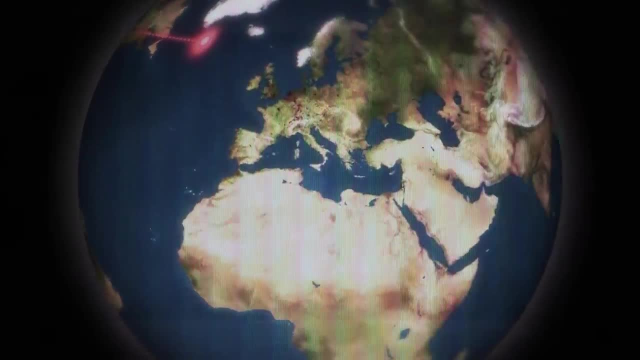 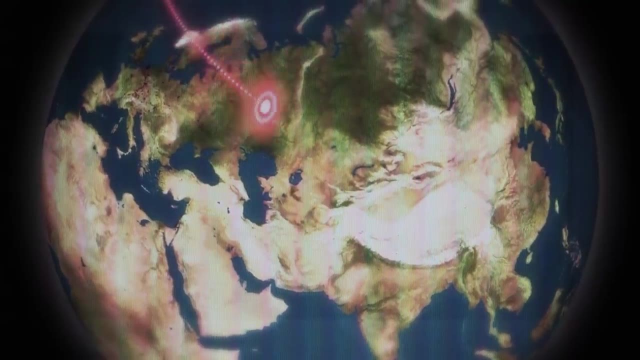 Like in 1983, the Soviet satellite-based early warning system detected the launch of an intercontinental ballistic missile from the US, But the US hadn't launched anything. The Soviet system had confused sunlight reflecting off high-altitude clouds with a ballistic missile. 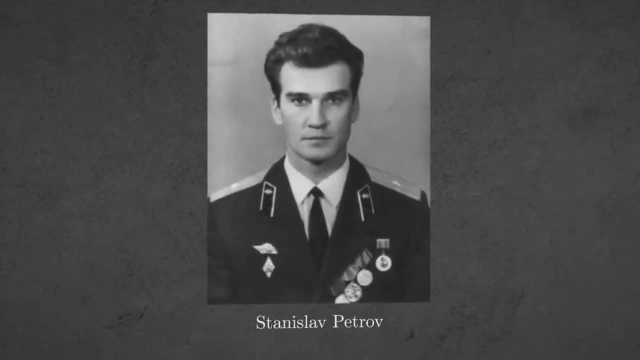 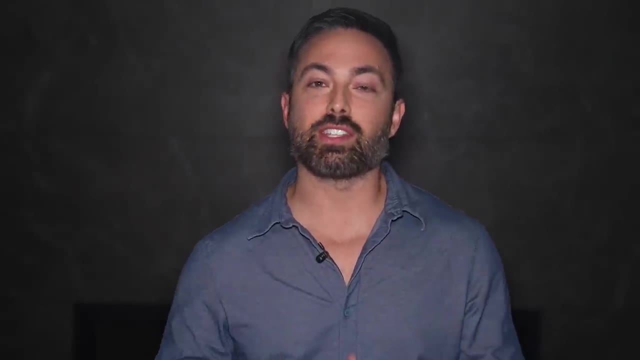 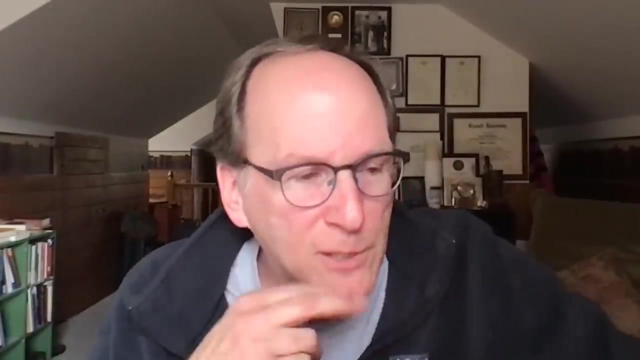 Thankfully, Stanislav Petrov, the Soviet officer on duty, dismissed the alarm. But this example shows the potential costs of a signal error and the importance of studying the effects of noise on those strategies. The word game sounds like it's a children's game or, you know, there's something, a misnomer. 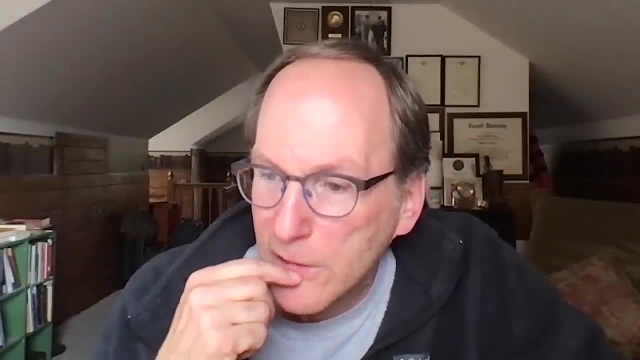 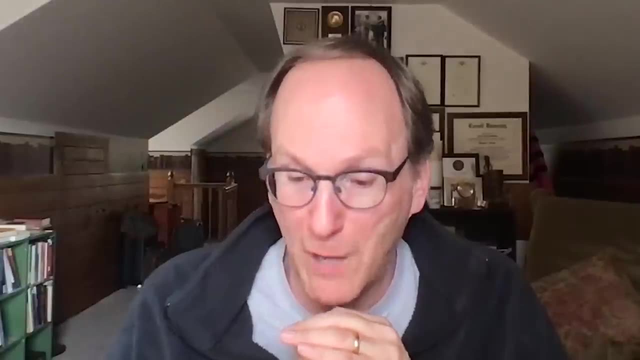 maybe in calling it game theory, because this is, these are life and death matters. obviously, As you mentioned that this came up in the Cold War. I mean, it could actually be life and death of the whole planet. We could annihilate human civilization. 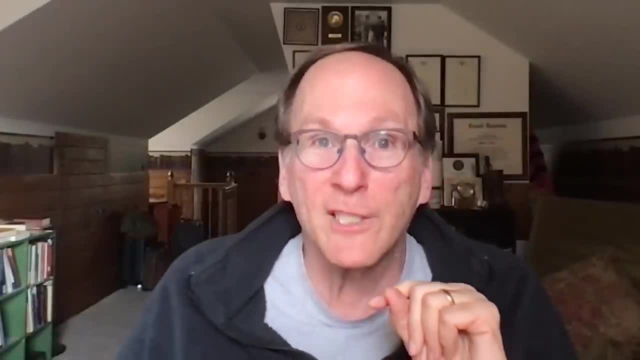 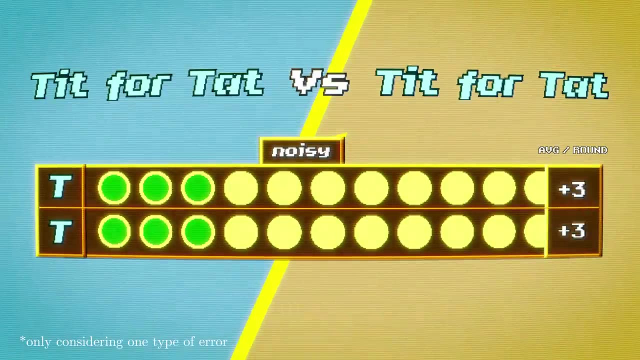 So these are not games In a way. they're not games In any kind of trivial sense. It's just the term that is used by mathematicians and theorists When tit-for-tat plays against itself in a noisy environment. both start off by cooperating. 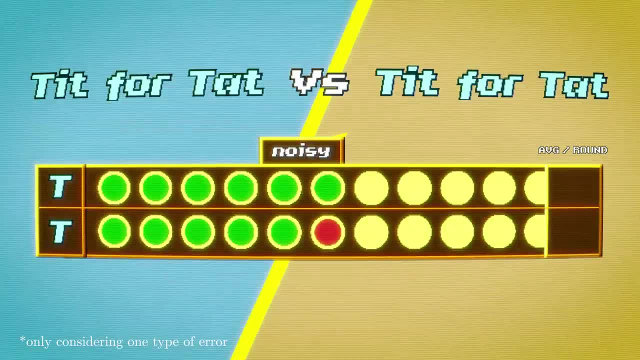 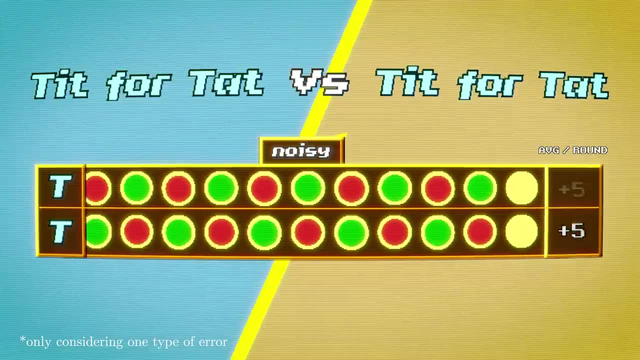 But if a single cooperation is perceived as a defection, then the other, tit-for-tat- retaliates and it sets off a chain of alternating retaliations. And if another cooperation is perceived as a defection, then the rest of the game is. 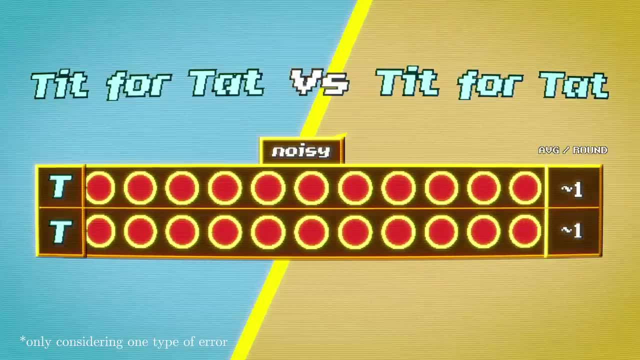 constant mutual defection. Therefore in the long run both would only get a third of the point. So in the long run both would only get a third of the point. So in the long run both would only get a third of the point. 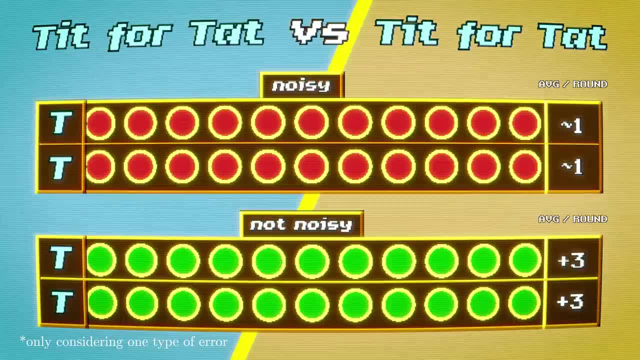 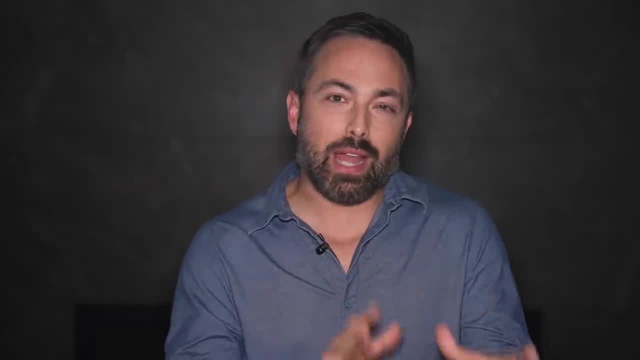 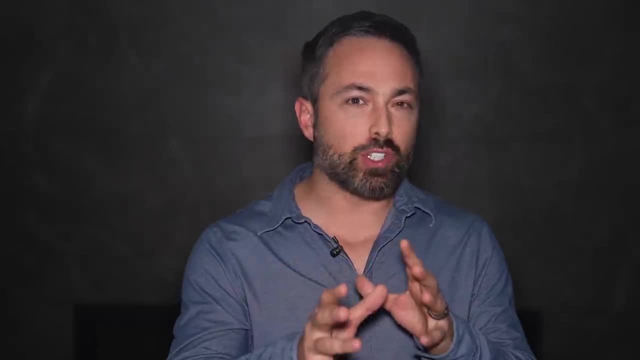 But there were some points they would get. in a perfect environment, Tit-for-tat goes from performing very well to performing poorly. So how do you solve this? Well, you need a reliable way to break out of these echo effects, And one way to do this is by playing tit-for-tat, but with around 10% more forgiveness. 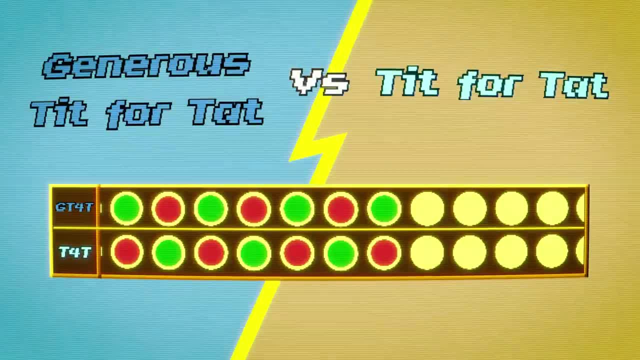 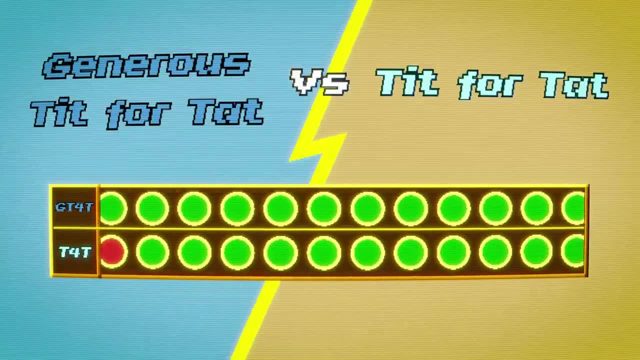 So, instead of retaliating after every defection, you only retaliate around nine out of every ten times. This helps you break out of those echoes while still being retaliatory, but also giving enough to not be taken advantage of. And so we also ran the tournament with. 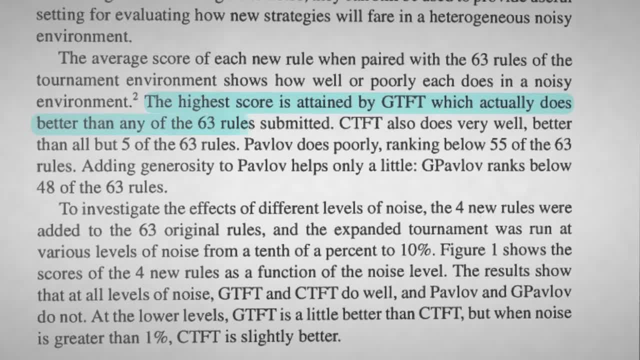 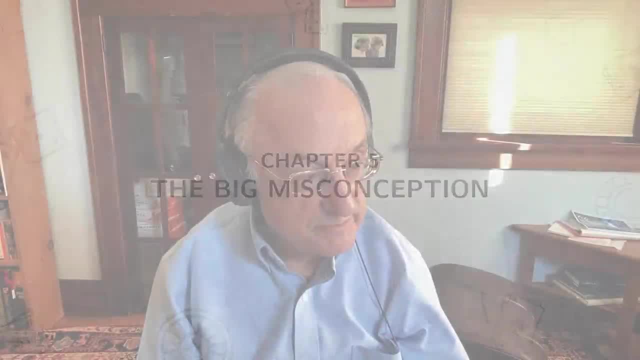 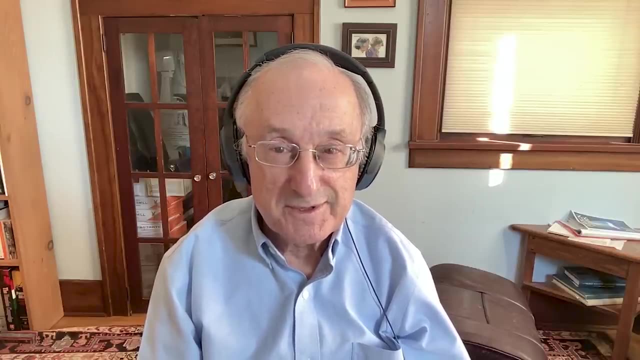 noise and generosity, And that did quite well. My favorite example is Tit, for Tat does really well, but it could never do better than the player it's playing with. I mean, think about it By design. all they can do is lose or draw. 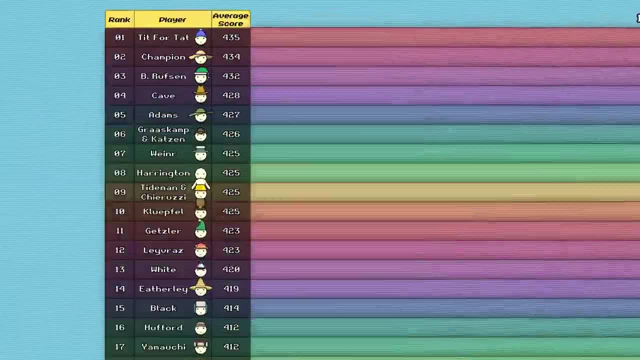 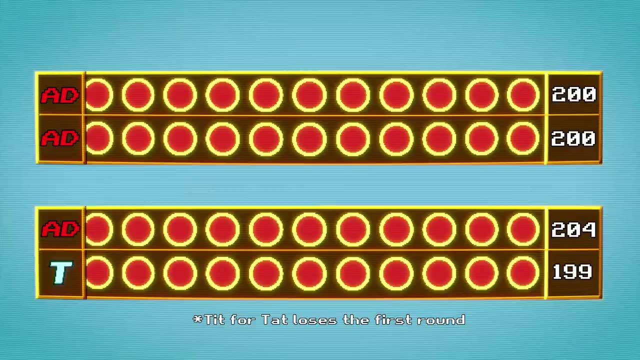 And yet when the results of all interactions are tallied up, they come out ahead of all other strategies. Similarly always: defect can never lose a game. It can only draw or win, But overall it performs extremely poorly. This highlights a common misconception, Because for many people, when they think about winning, 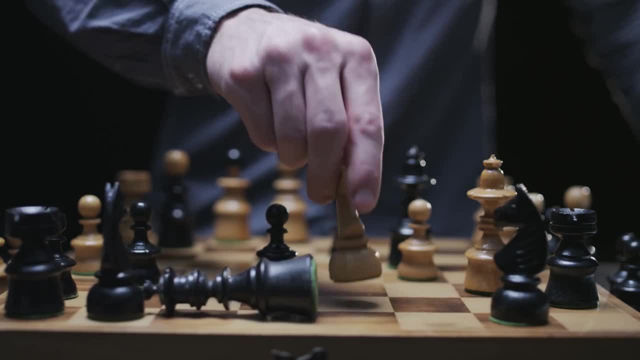 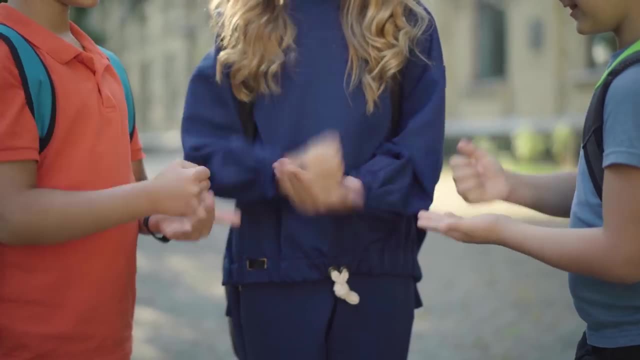 they think they need to beat the other person In games like chess or poker. this is true, since one person's gain is necessary And it's not necessarily another person's loss. So these games are zero-sum, But most of life is not zero-sum. To win, you don't need to get your. 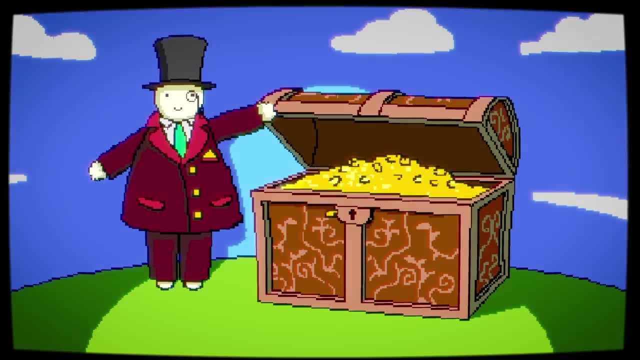 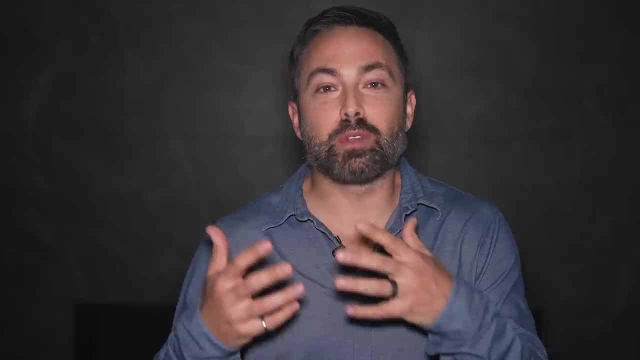 reward from the other player. Instead, you can get it from the banker Only in real life, the banker is the world. It is literally everything around you. It is just up to us to find those win-win situations and then work together to unlock those rewards. 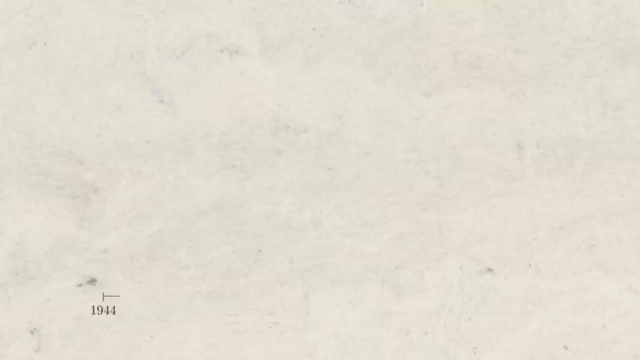 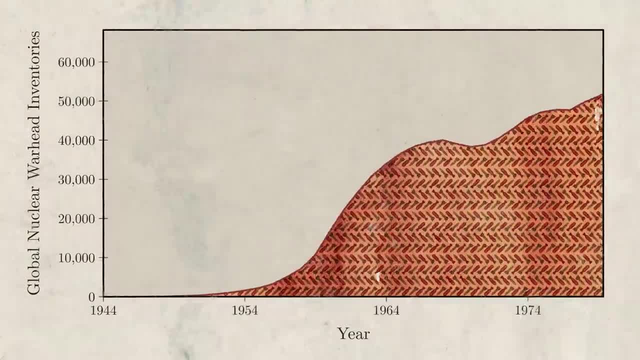 From 1950 to 1995, we had a lot of experiences in this realm. From 1950 to 1995, we had a lot of experiences in this realm. In 1986, the US and Soviet Union had trouble cooperating and both kept developing nukes. But then, from the late 80s onwards, they started reducing their nuclear stockpiles. They too had learned how to resolve conflict. Rather than making an agreement to abolish all nuclear arms at once and essentially turning it into a single prisoner's dilemma, they would disarm slowly a small number of nukes. 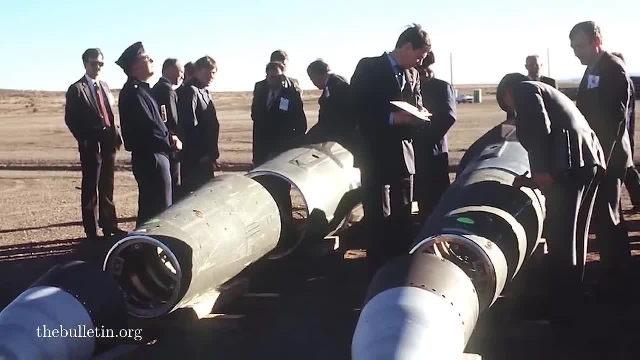 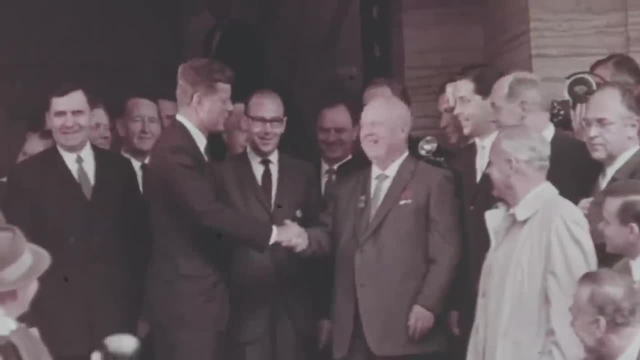 each year, and then they'd check each other to see that they had both cooperated, and then repeat the year after and the year after that, all along checking to ensure mutual cooperation. In the more than 40 years since Axelrod's tournaments, researchers have continued to. 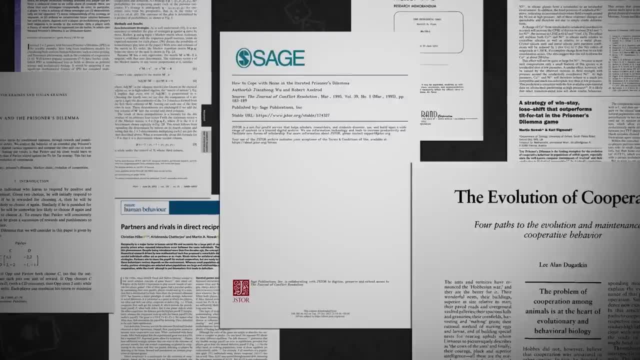 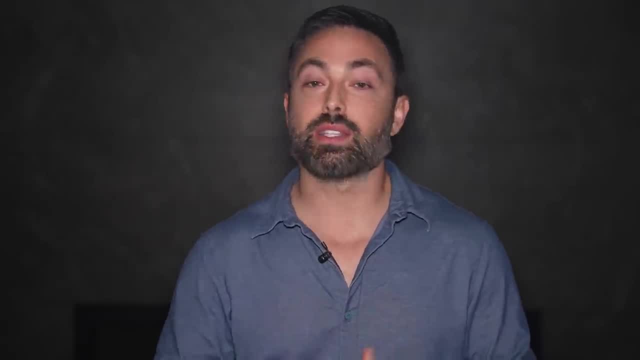 study which strategies performed best in a variety of environments. In doing so, they varied everything from payoff structures to strategies, to errors and more. Some even allowed the strategies to mutate, While tit-for-tat- or generous tit-for-tat- doesn't always come out on top. Axelrod's. 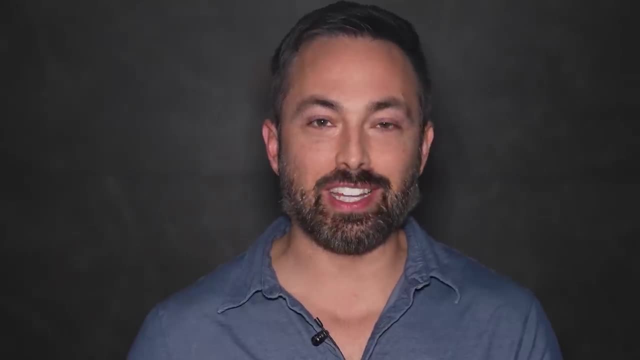 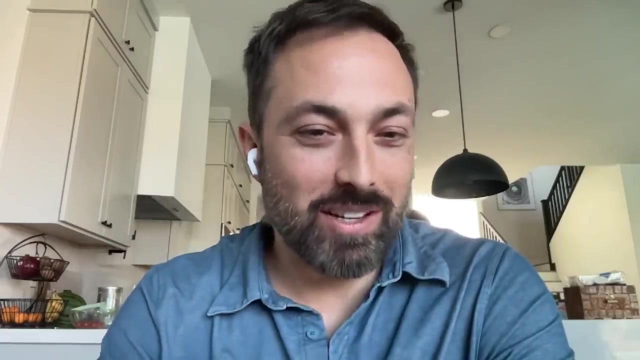 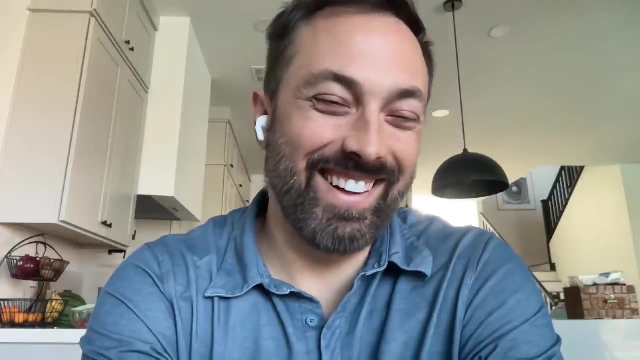 main takeaways still hold: Be nice forgiving, but don't be a pushover. Can I ask you, why did Anatole Rapoport submit tit-for-tat? Well, the reason was because I asked him to And he wrote saying, yeah, I'm willing to do that. 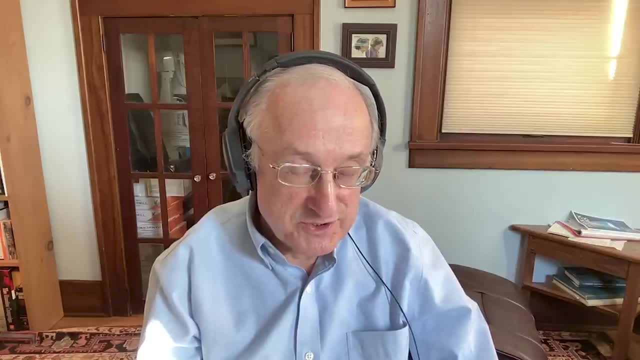 But I just want to be clear. I'm not sure that this is really such a good idea. I don't. he was a peace researcher And I think his own inclinations were to be much more forgiving and maybe and not be so provokable. 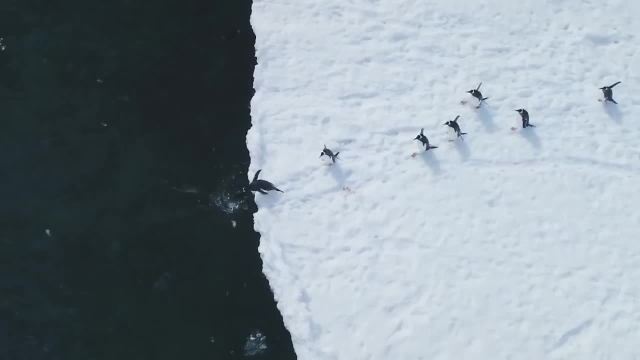 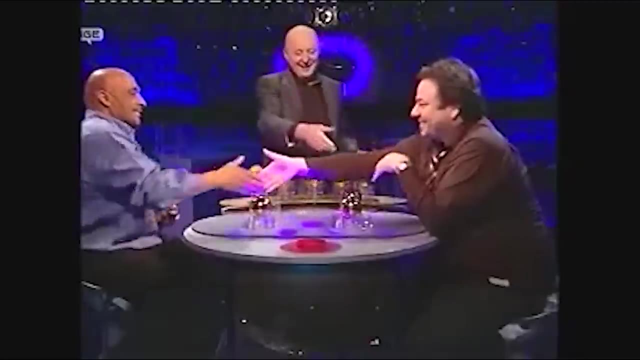 What I find fascinating is that one of the main things that sets life apart from non-living things is that life gets to make decisions. We get to make choices, choices that don't only change our future, but also the future of those we interact with. 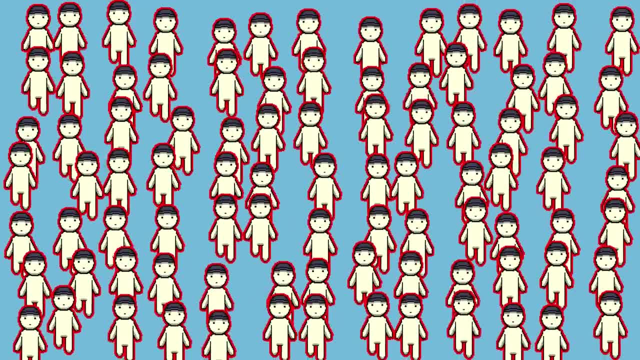 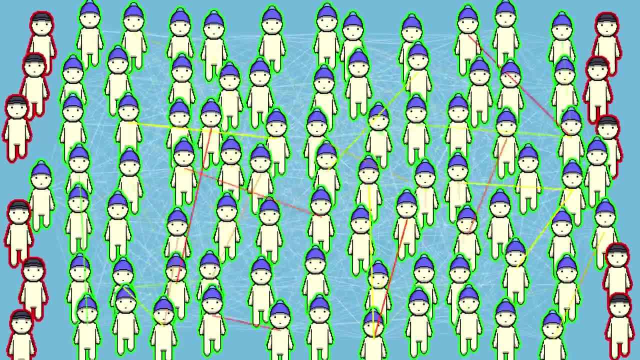 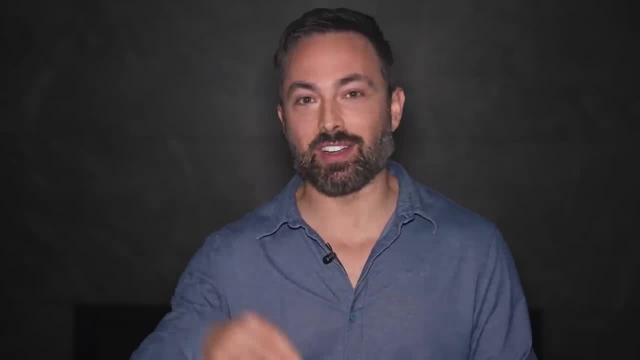 See, It's often the environment that shapes the player, that determines who does well, But in the long run, it is the players that shape the environment. So let's play a game, the game of life, and make your choices wisely, because their impact. 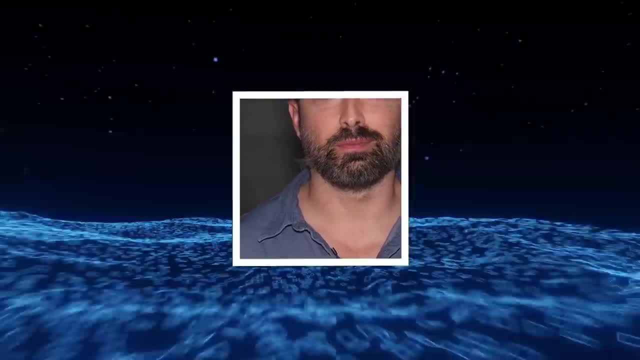 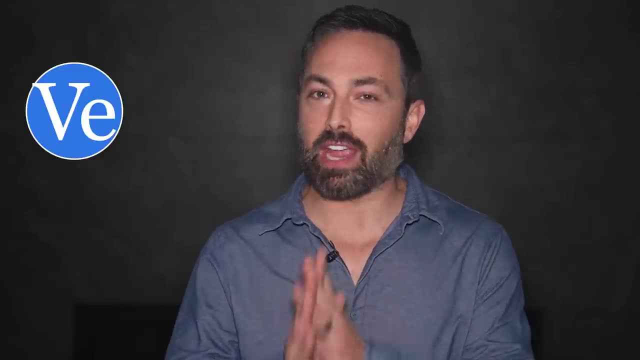 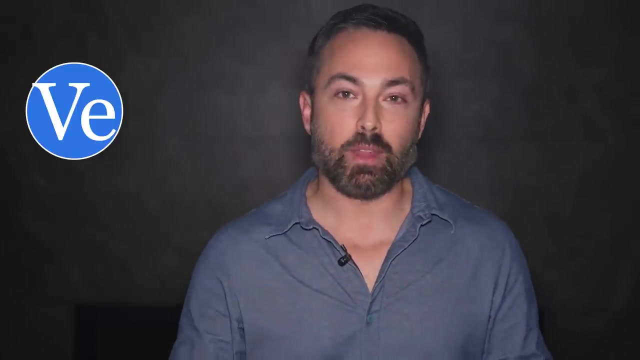 may reach further than you think. Using the right strategy matters, but figuring out the best strategy isn't easy. It requires critical thinking and innovative solutions, like Axelrod's tournaments. If you're looking for an easy way to build your problem-solving skills, then check out. 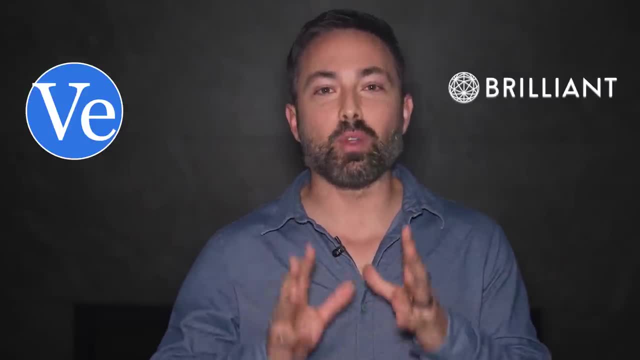 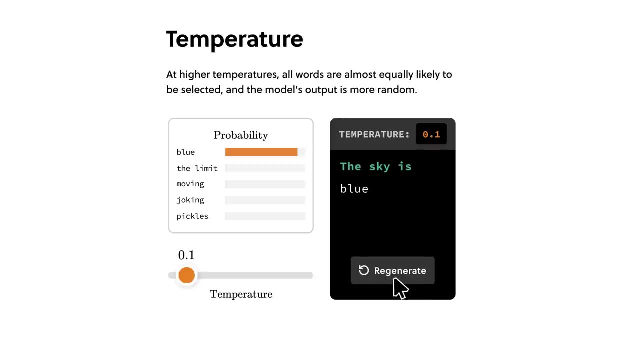 this video's sponsor, Brilliant. Brilliant will help make you a better thinker in everything from math and data science to programming technology, you name it. You can start right now, for free, straight from your device. the device you're watching this on.